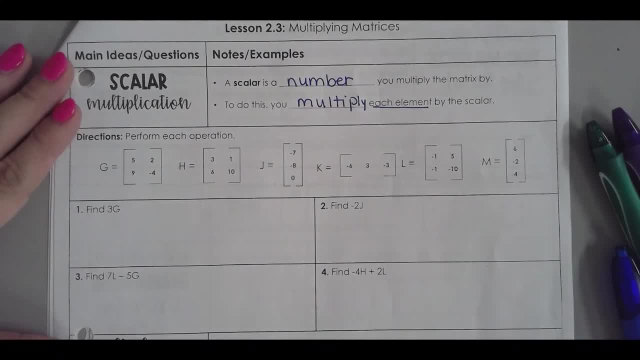 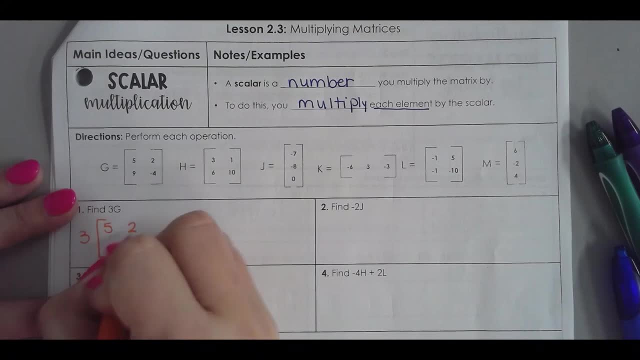 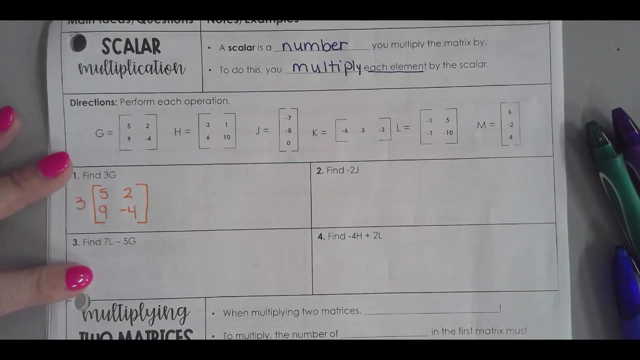 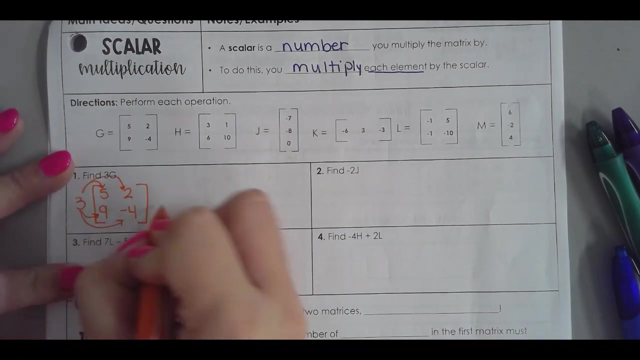 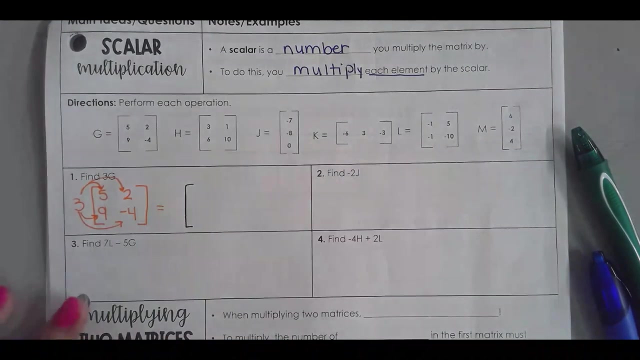 numbers that are in front of a matrix. you just multiply each element by the scalar G, You're doing three times matrix G And essentially what you're doing is distributing that three Three. So we would do three times five, which is 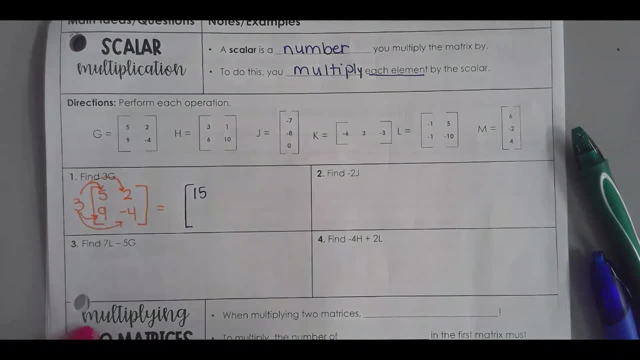 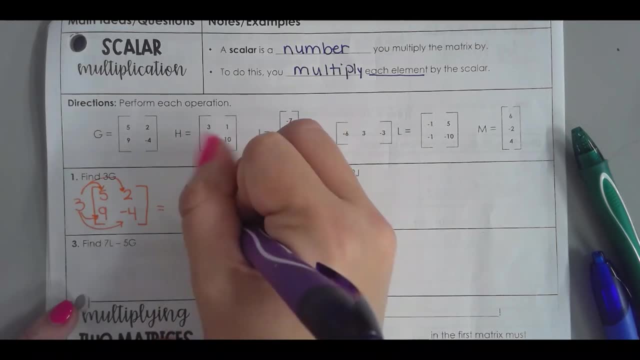 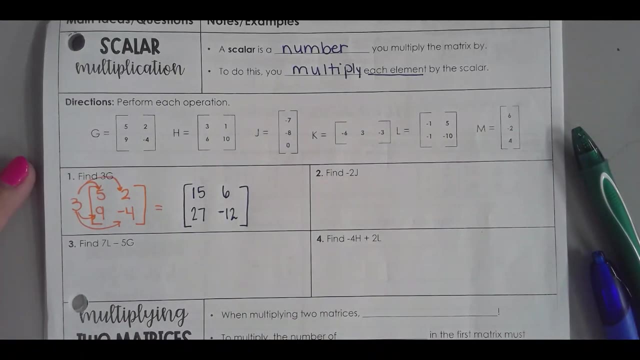 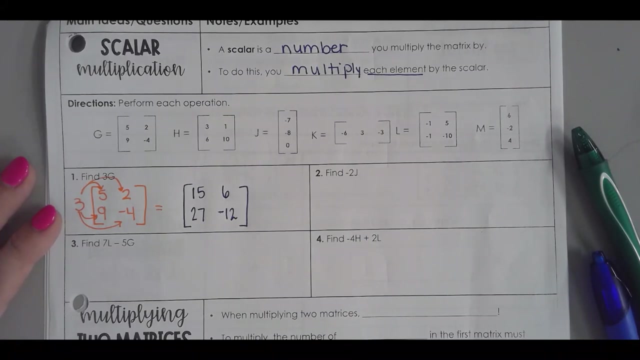 what? Yes, Three times two, Six, Three times nine And three times negative four, Negative twelve. Good, That part is, I would say, easy. Yes, I'm going to see like matrix H plus three. You cannot add a single. 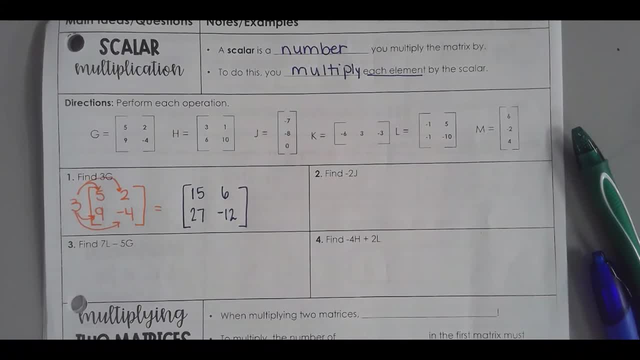 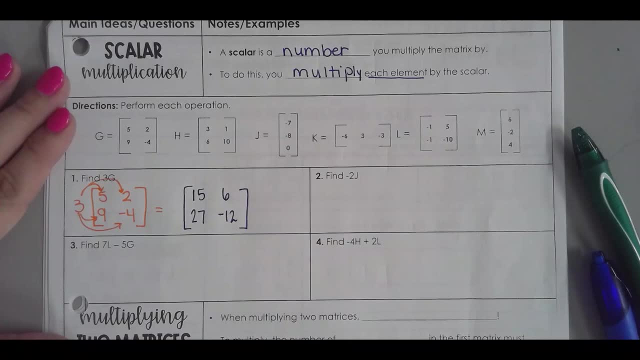 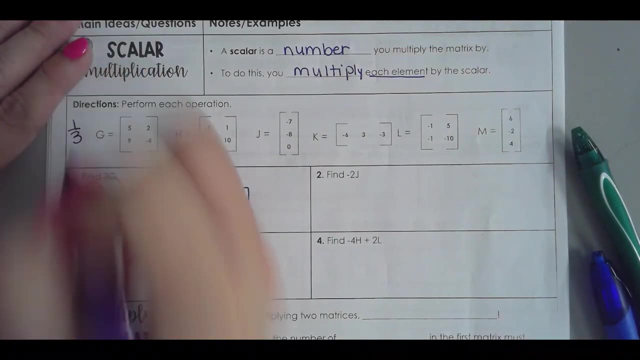 number. You can't add a number to a matrix, But you can multiply by a number. Can you divide? Yeah, I'm not going to say G divided by three, But what I could do is say one third G, One third Multiplying. 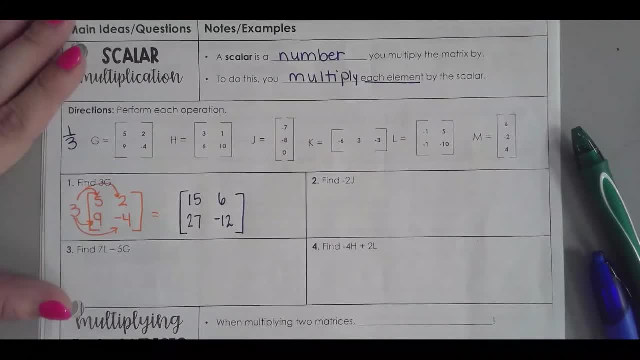 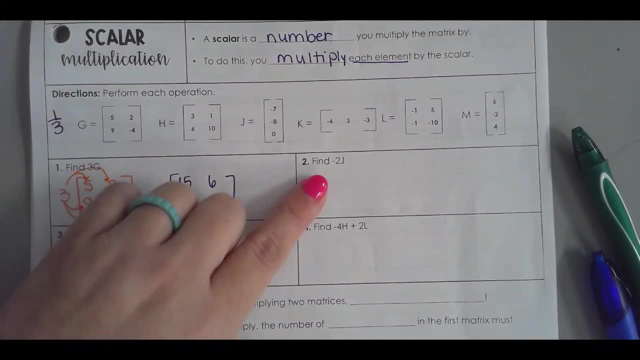 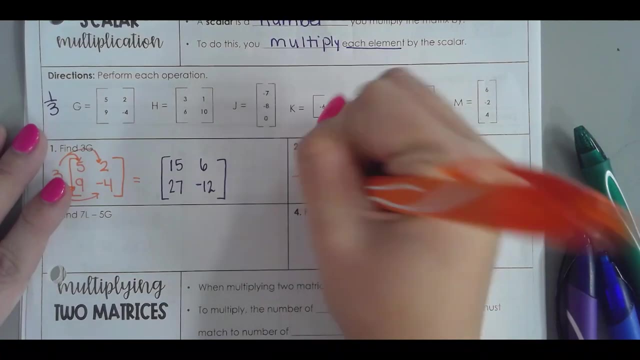 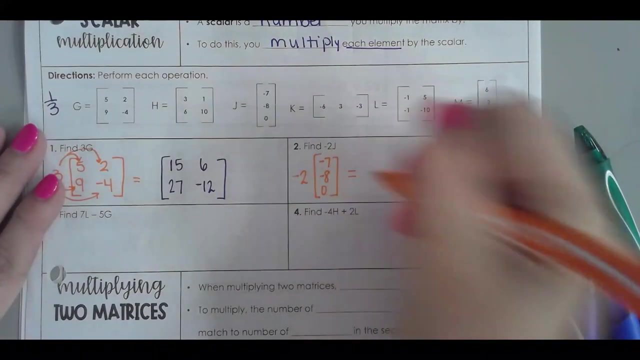 by one third is the same as dividing by three. Multiplying by one half is the same as dividing by two. Okay, So number two: Negative two, Two J. So negative two J is that matrix And in the calculator, 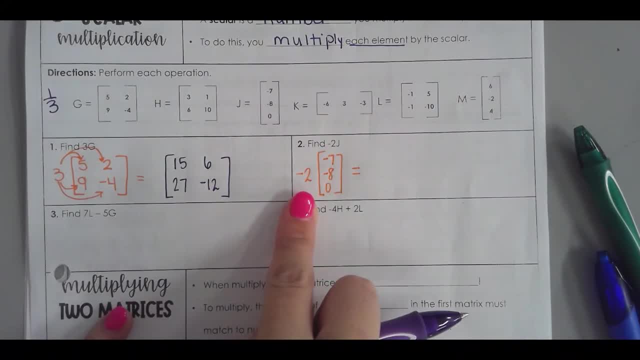 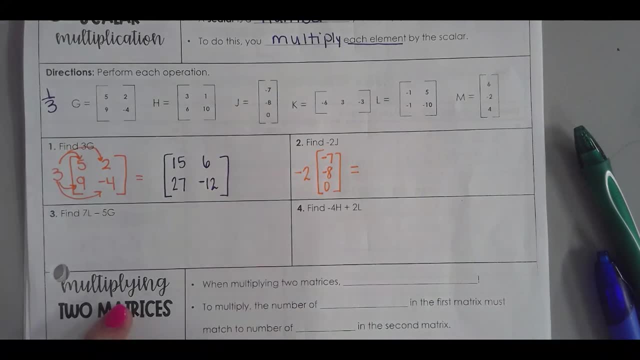 again. it probably would take you more time to type it in than just to do the math. But you can type in a number and then type in a matrix right beside of it And it'll do the calculations. Negative two times negative seven is: 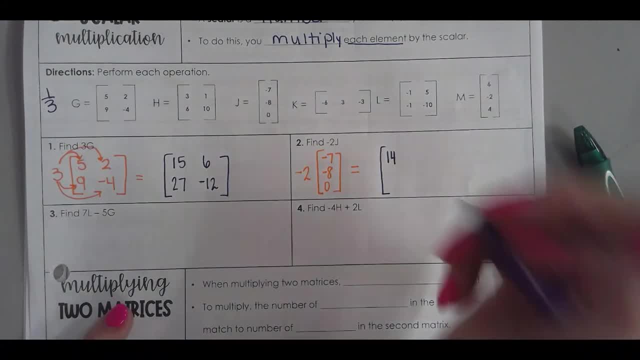 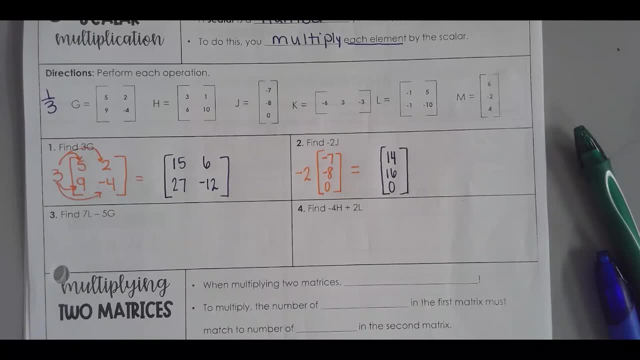 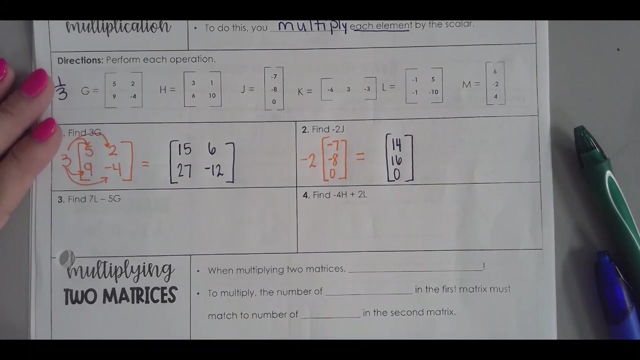 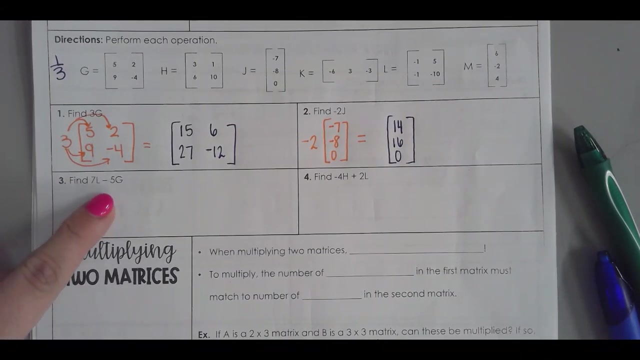 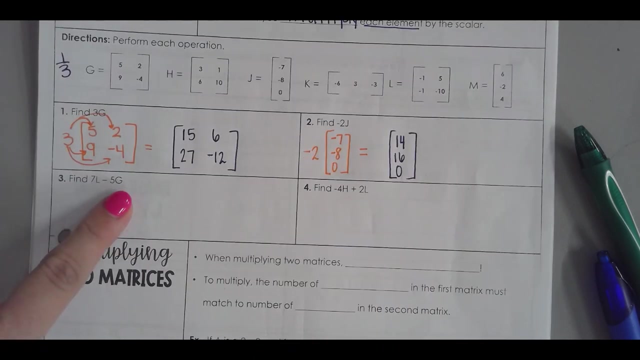 fourteen Negative, two times negative. eight is sixteen And then zero. Number three is seven L minus five G. So what we're doing is multiplying matrix L by seven, multiplying matrix G by five and then subtracting those two matrices. Now I really 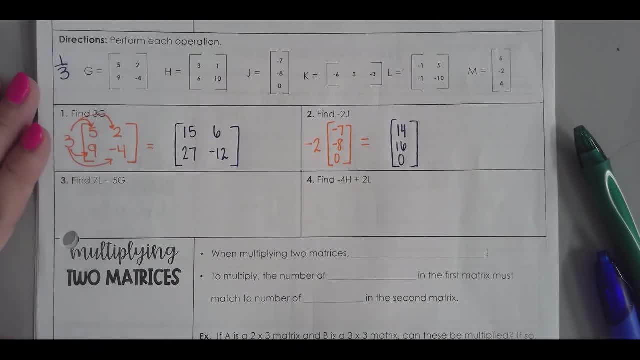 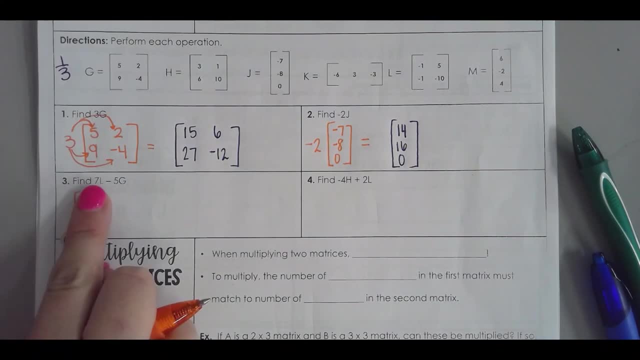 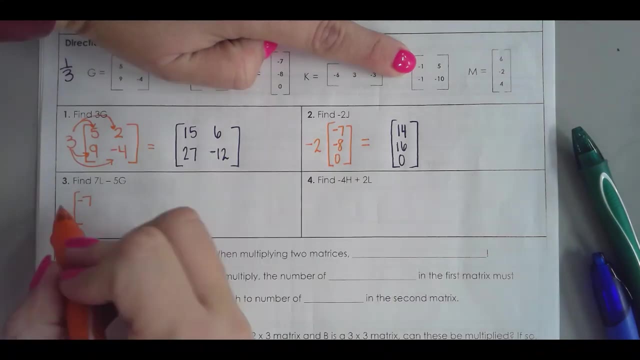 didn't leave you enough room to show all of your work, So I'm just going to go ahead and kind of do seven times L. Okay. So seven L, Seven times negative. one is negative. seven. Seven times five is thirty-five. 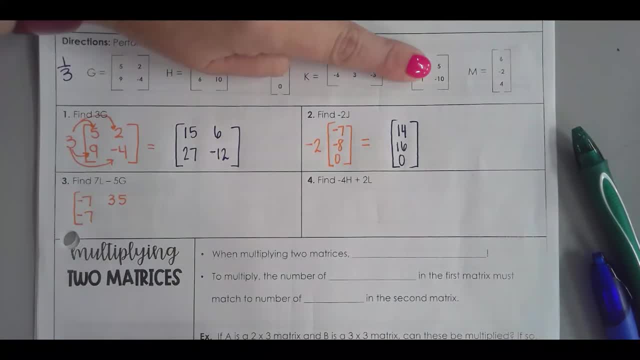 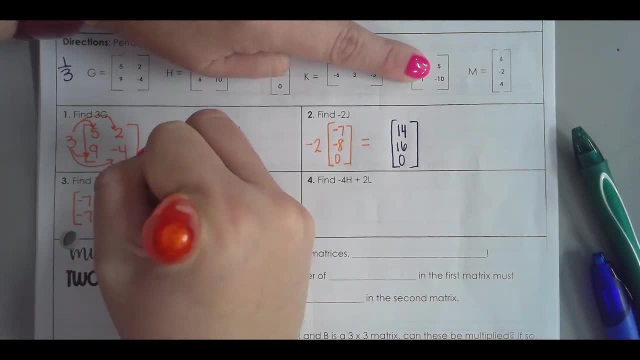 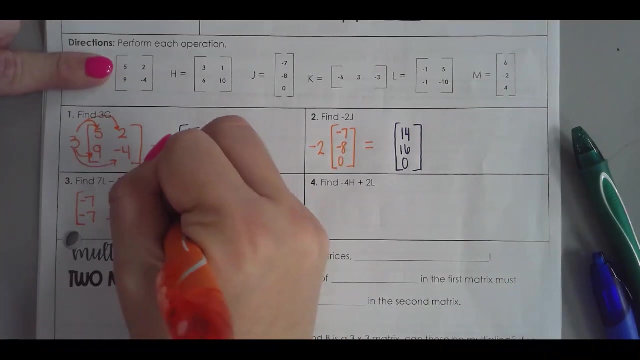 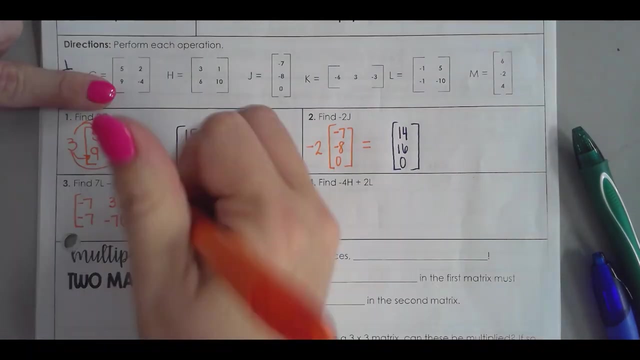 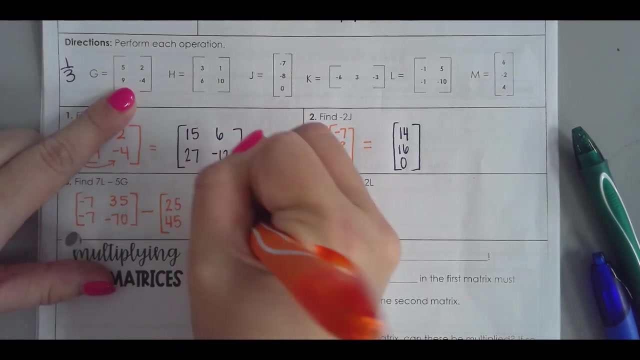 Negative seven and seven times negative ten negative seventy minus five G. So five times five is twenty-five. Five times two, Five times nine, Forty-five And five times negative four, Negative Negative: twenty. And then I can: 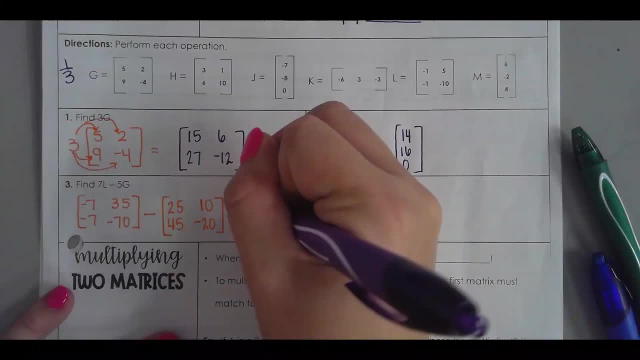 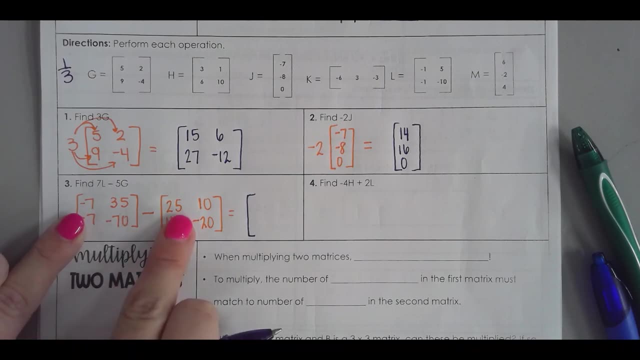 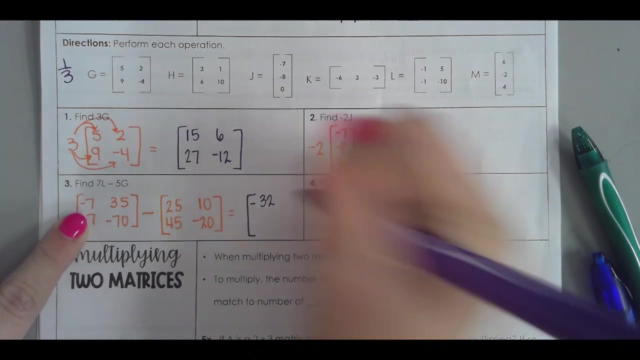 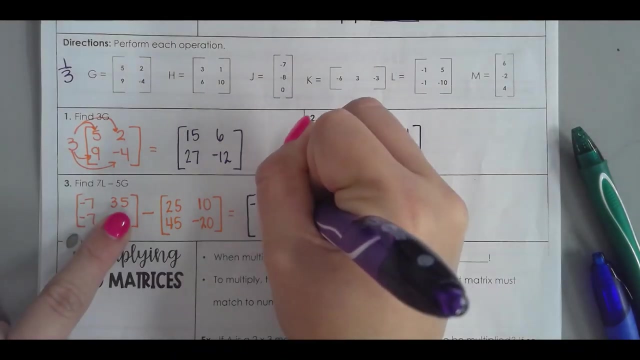 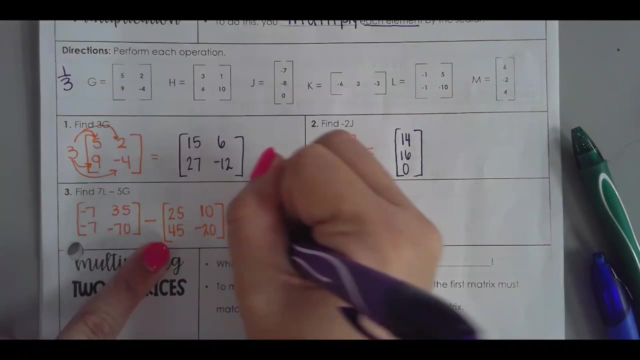 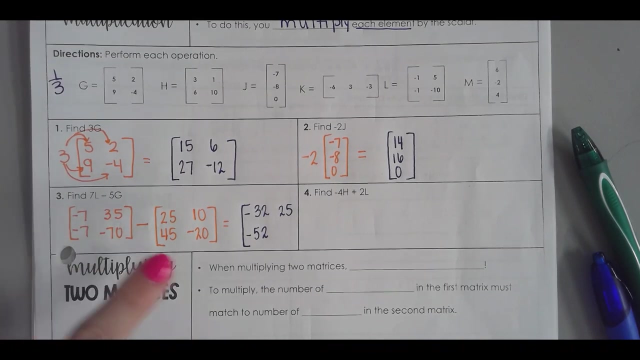 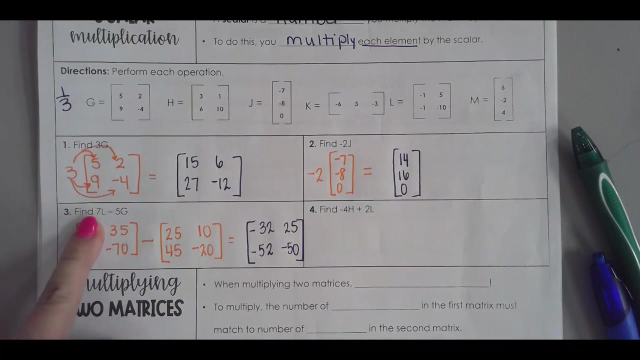 subtract them: Negative seven minus twenty-five, Negative thirty-two. Thirty-five minus ten is twenty-five. Negative seven minus forty-five, Negative fifty-two. And negative seventy minus negative twenty, Negative fifty. And again. you can type this in the calculator: 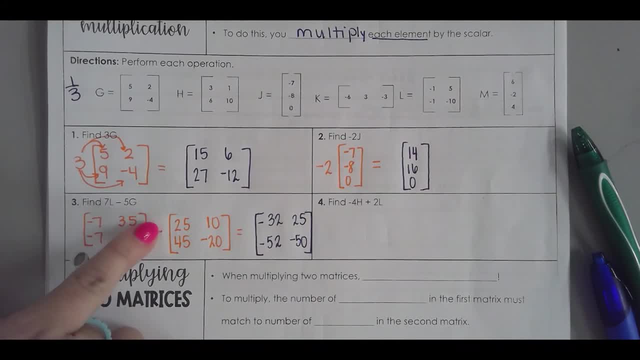 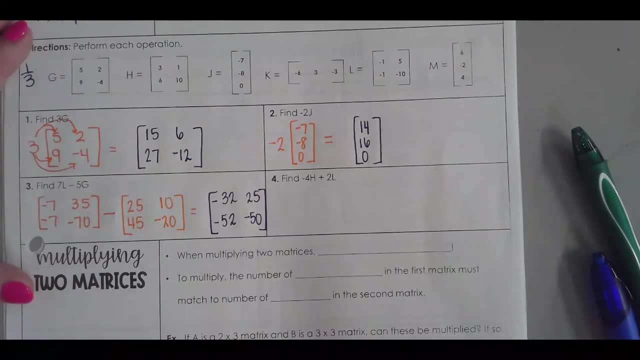 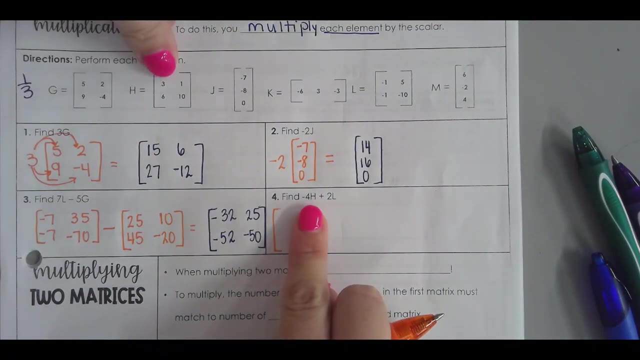 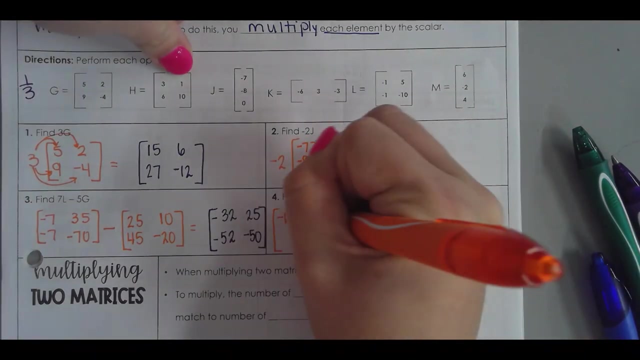 You can type in a seven and then matrix L minus five, matrix G: Alright, Let's do number four: Negative four. Negative four: H. So negative four times three is negative twelve. Negative four times one is negative four. 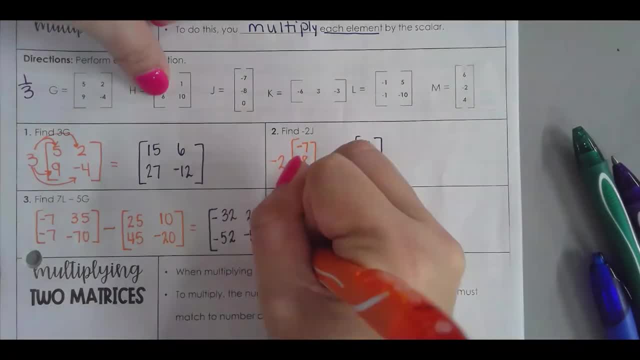 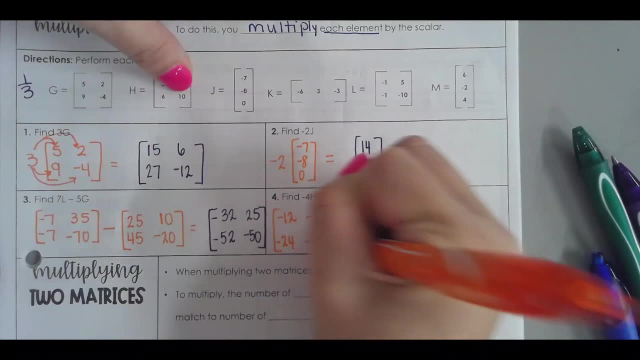 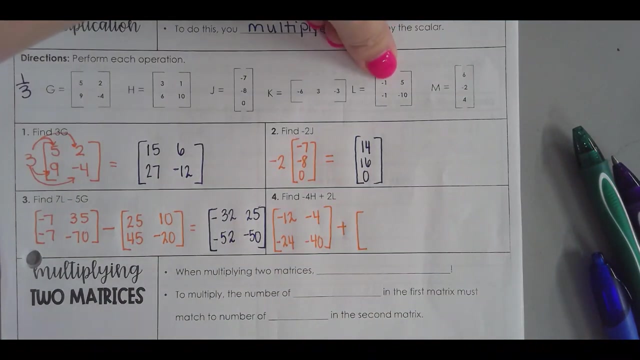 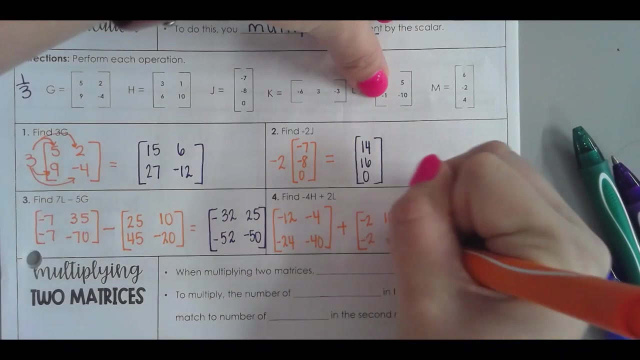 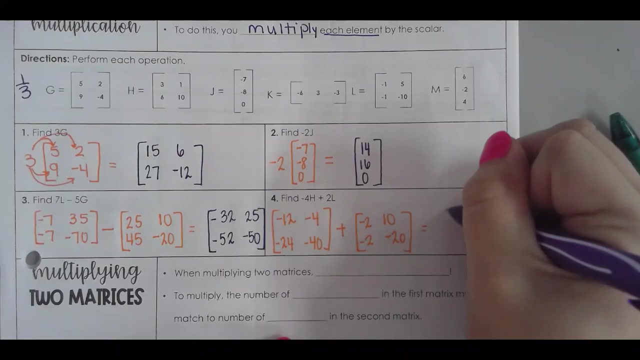 Negative four times six is negative twenty-four And negative four times ten. Negative forty Plus two. L Two times negative. one is negative two. Two times five is ten. Negative two. Negative twenty, And then when I add those I get negative fourteen. 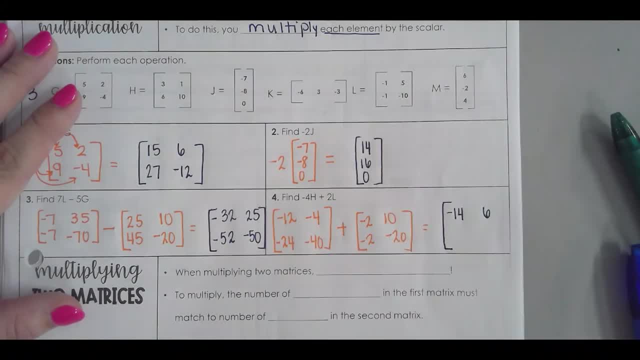 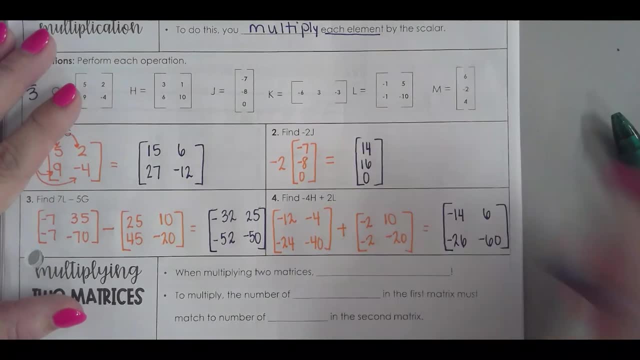 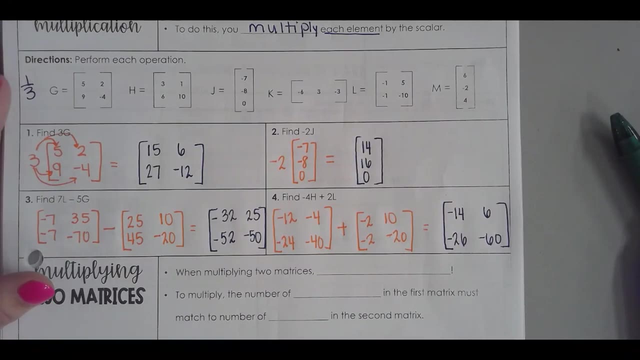 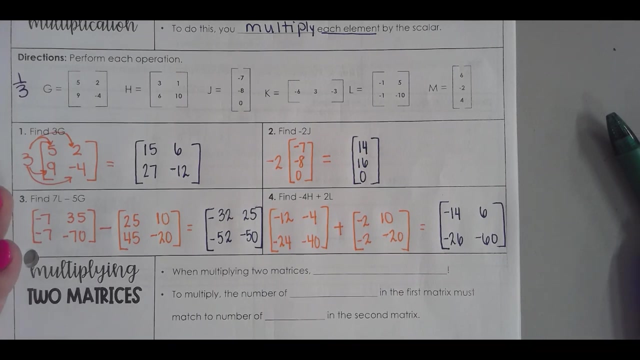 Six, Negative twenty-six And negative sixty. Any questions? If you can distribute, that's all this is. Then come back to the next question. Okay, So then comes multiplying two matrices by each other. It's not a number times a matrix. 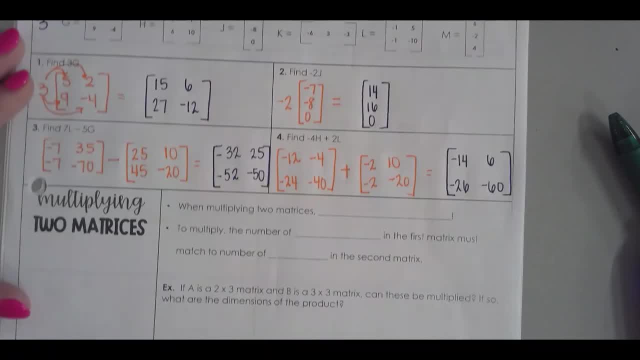 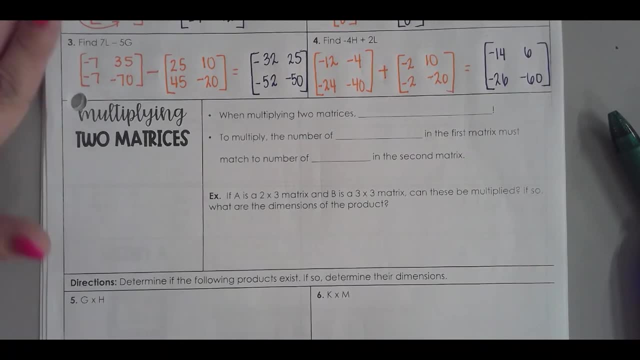 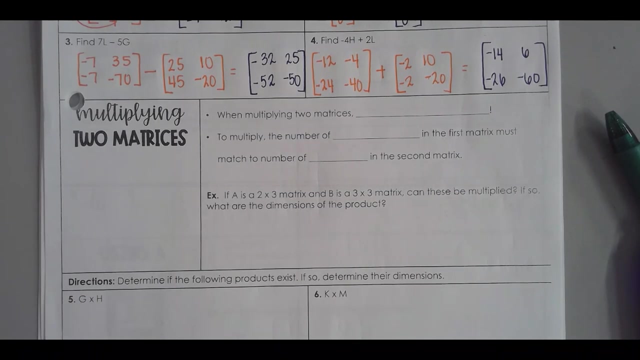 It's a matrix times a matrix And there are some rules to be able to do this. It is different than adding and subtracting. The big rule for adding and subtracting is that both matrices have to have the same dimensions. That's not. 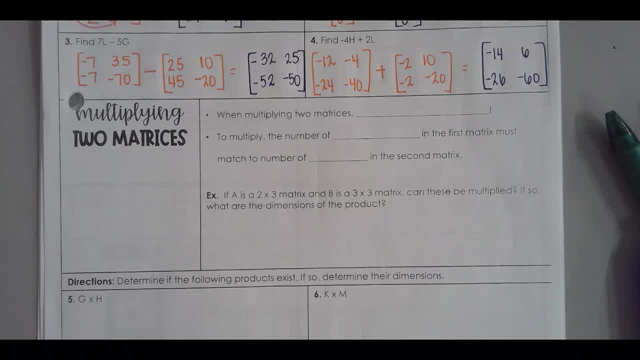 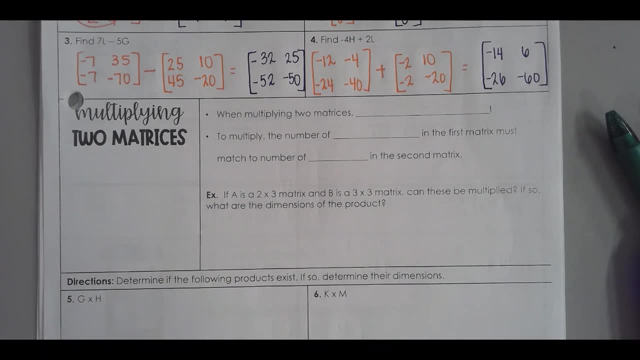 the case when we multiply. Sometimes, if they have the same dimensions, it doesn't even work at all, And I want to show you how to figure out if it's even possible. If you try to type it in the calculator and it's one that doesn't. 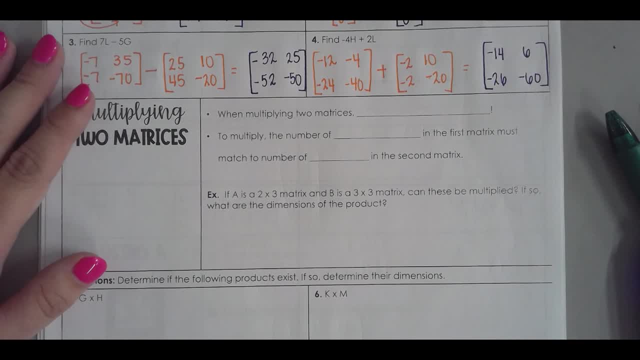 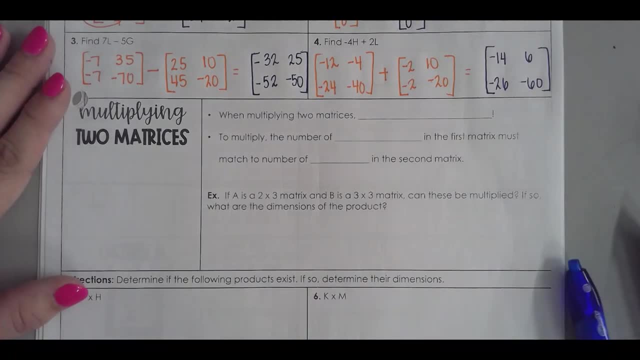 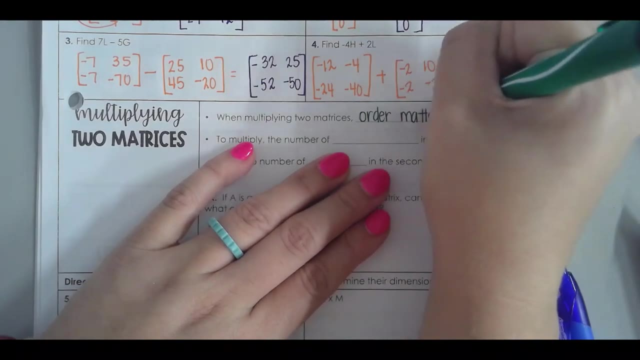 work. the calculator will give you an error, So it would tell you that it doesn't work. So another thing: when you multiply two matrices, order matters, So the order that you write your matrices matters. That's different than multiplying. 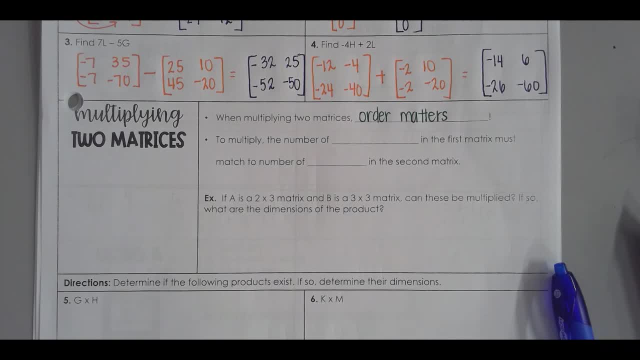 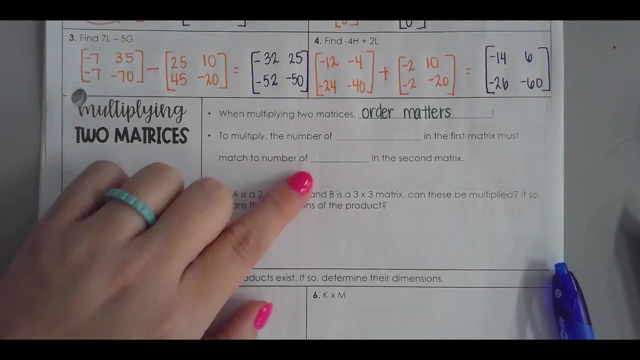 regular numbers. Two times three is the same thing as three times two, But matrix A times B will not give you the same answer as B times A. So the order matters. And then here's the other thing: To multiply the number of columns. 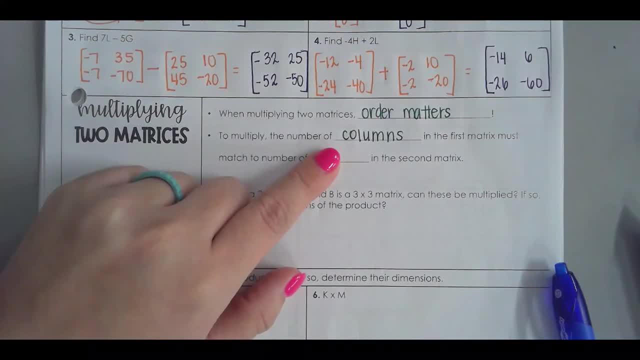 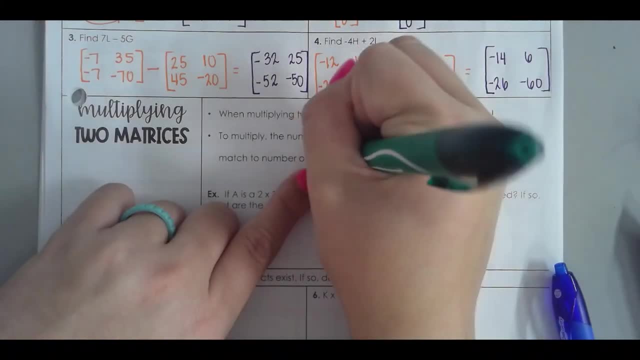 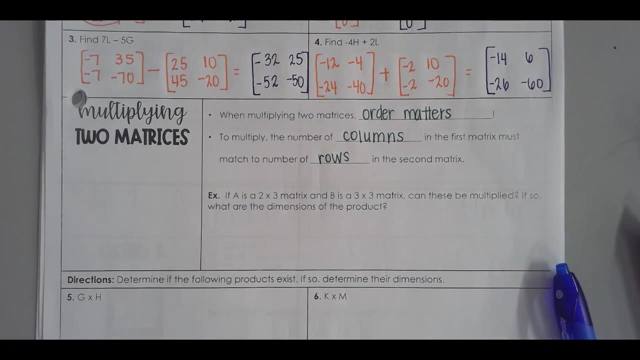 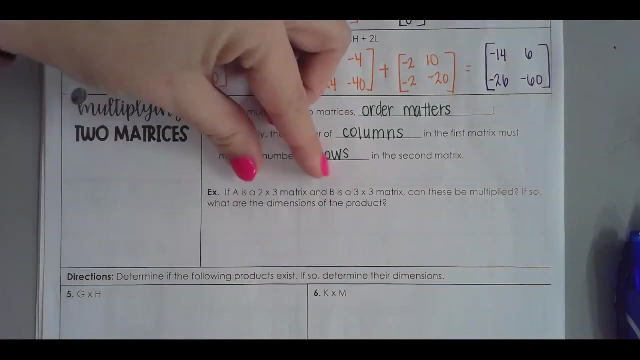 in the first matrix must match the number of rows in the second matrix, And there's a really easy way to see that. You don't have to think: okay, number of columns, number of rows. it's really easy, So I'm going to show you how. 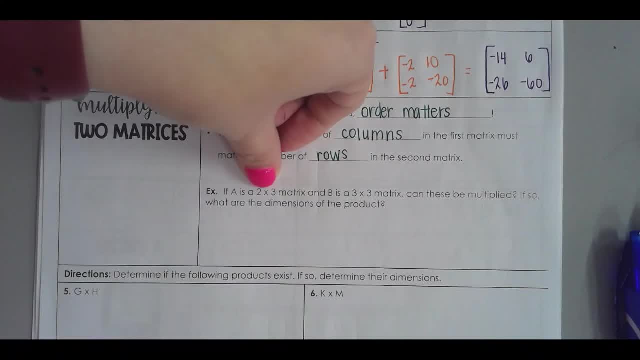 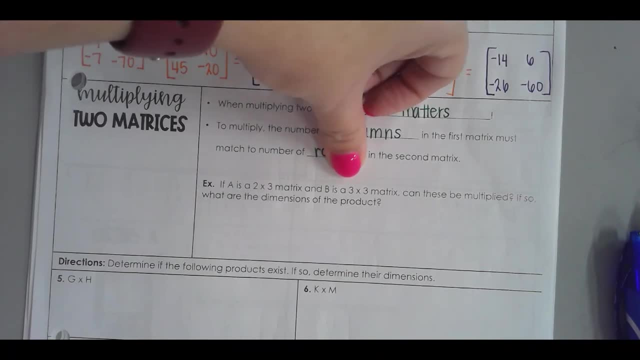 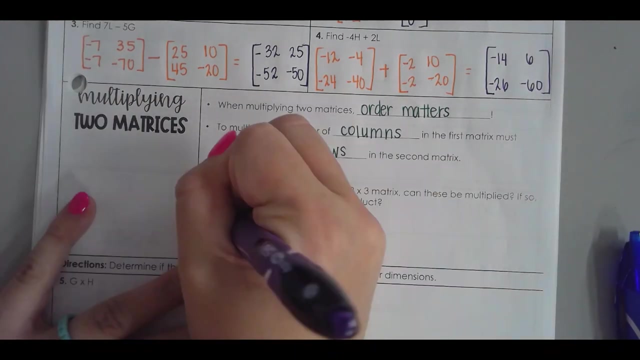 Matrix A is a two by three matrix And B is a three by three. I put an example here. I want to know if they can be multiplied. So if we want to do A times B, We want to multiply matrix A first. 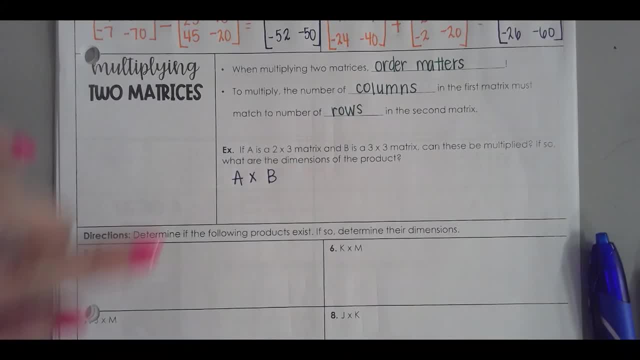 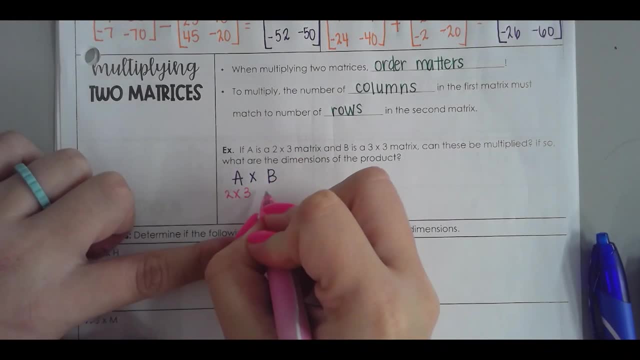 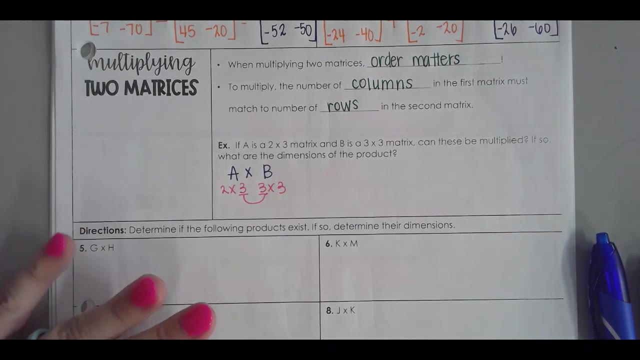 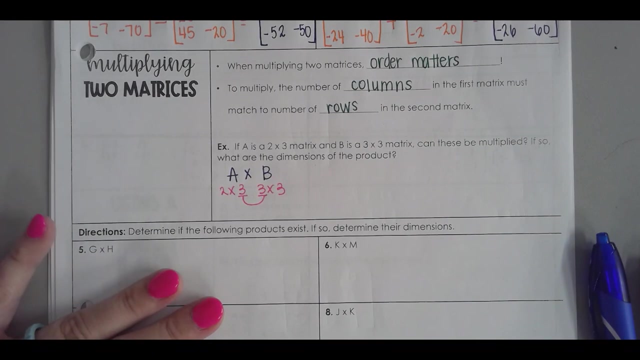 times matrix B. What are the dimensions of matrix A- Two by three And B- Three by three? You are looking at these middle numbers. You want those middle numbers to match. If the middle numbers match, then yes, you can multiply them. So do they? 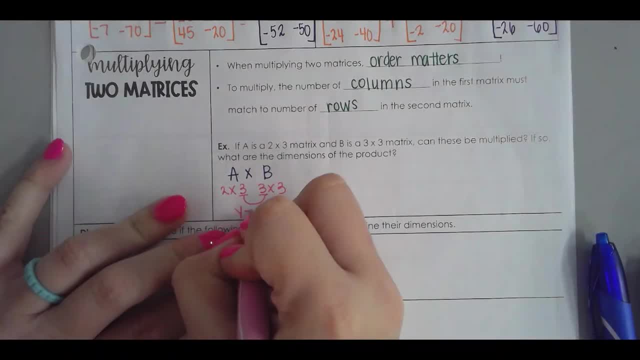 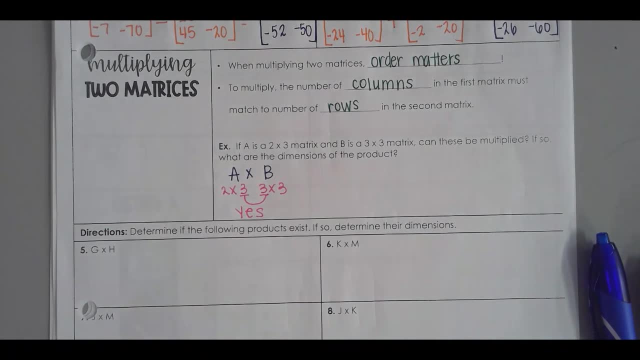 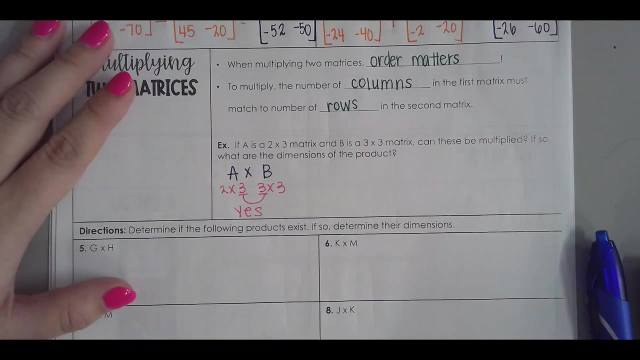 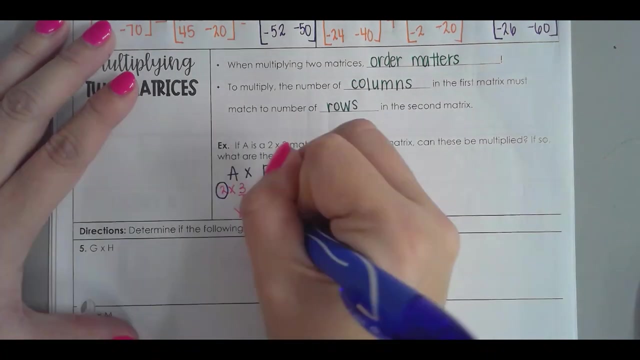 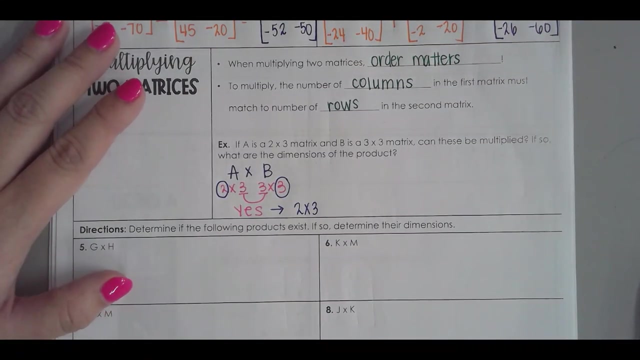 match? Yes, they do. Now, what else is neat is that this also tells us, when we multiply them, what size will my answer be? You look at these outside numbers. So my answer will be a two by three matrix. So this is matrix A. 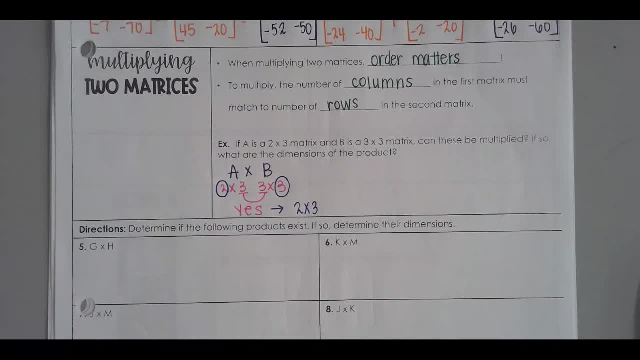 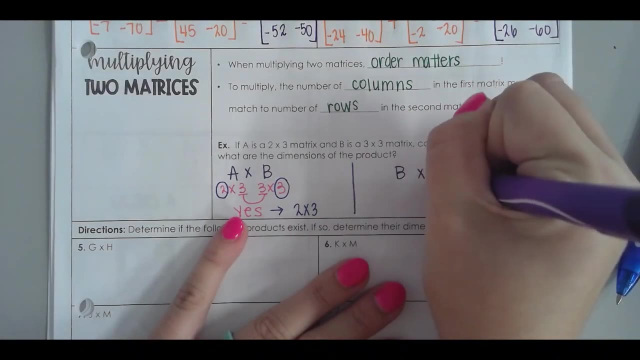 This is matrix B And I multiply them. If you were to type that in your calculator, your answer would be a two by three matrix. But what about flipping them? What if I wanted to do B times A? So if I wanted. 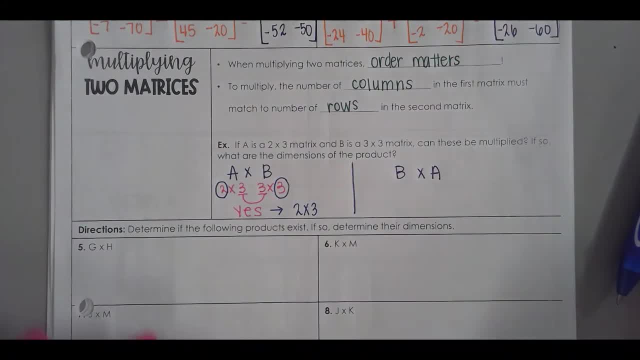 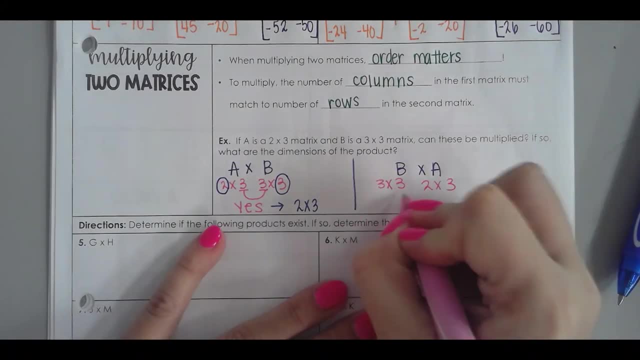 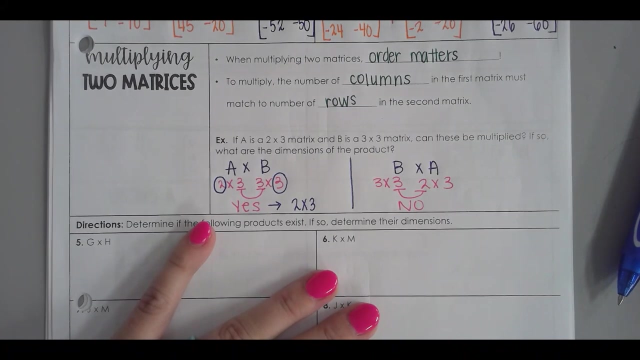 to flip-flop those. What are the dimensions of matrix B Two by three And A Two by three? Do the middle numbers match? No, So it's not even possible to multiply. Not only would you just get a different answer. 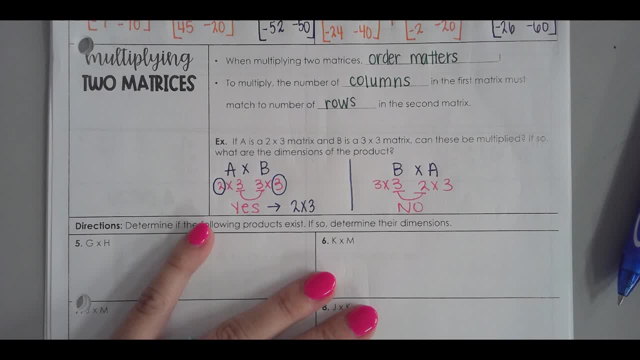 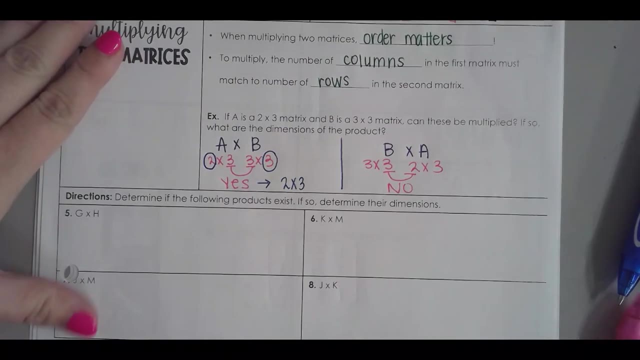 in this case it's not even possible to multiply them. Your calculator would give you an error and it would say invalid dimensions. The dimensions don't work. So in these four examples we're just going to see if it's possible. 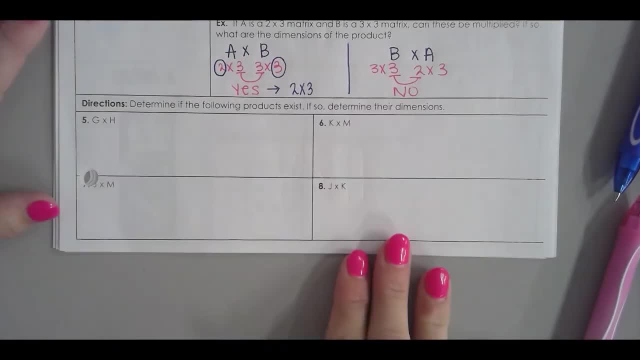 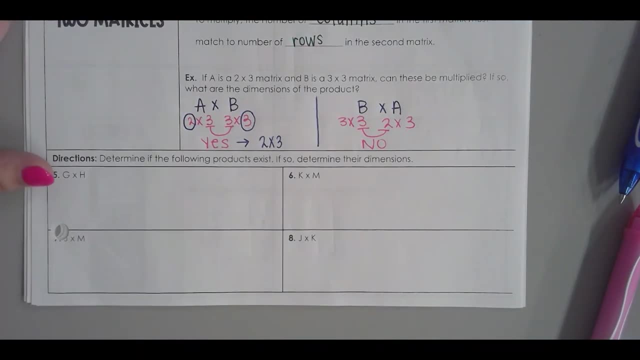 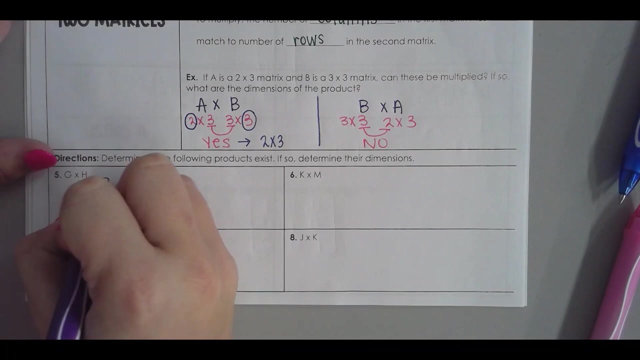 and if it is, what are the dimensions of my answer? Alright, so these are referring to the matrices at the top of your page. So G Is a? what Two by two? H is a Two by two. Does it work? 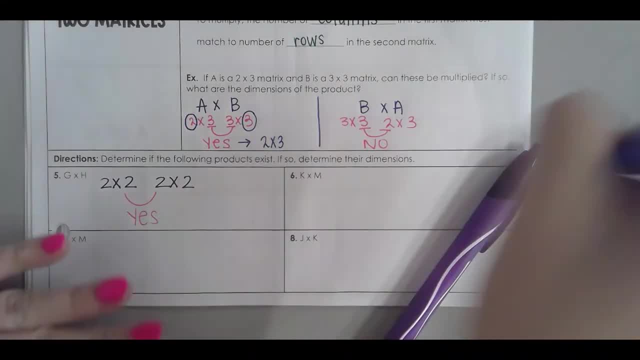 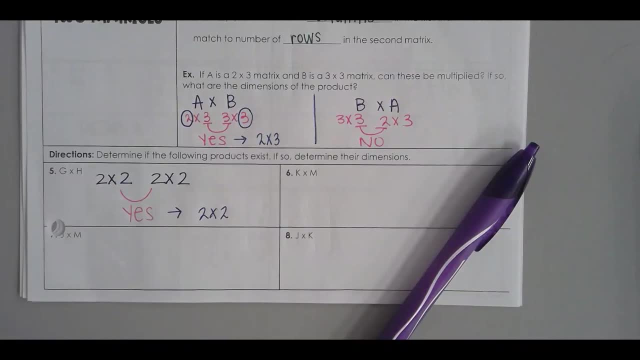 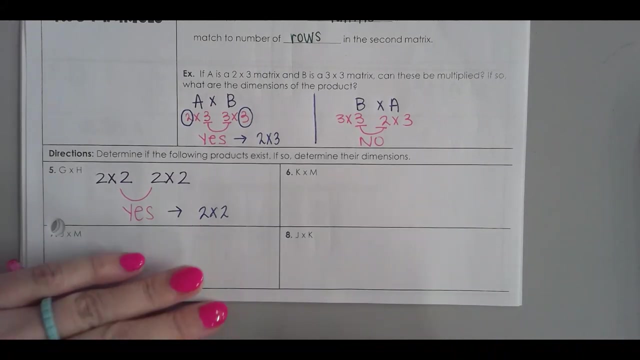 Yep, And my answer is a. It's a two by two Square matrices. if you take a three by three times a three by three, you're going to get a three by three. Alright, matrix K is a One by three. 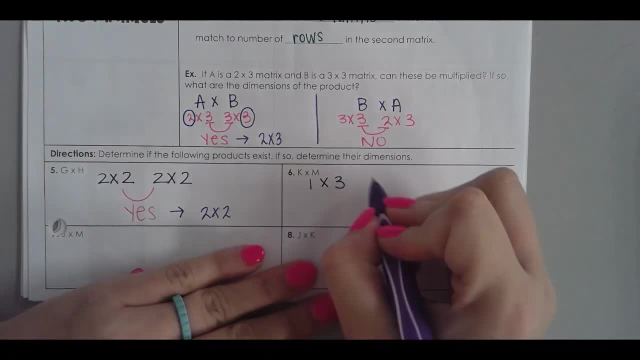 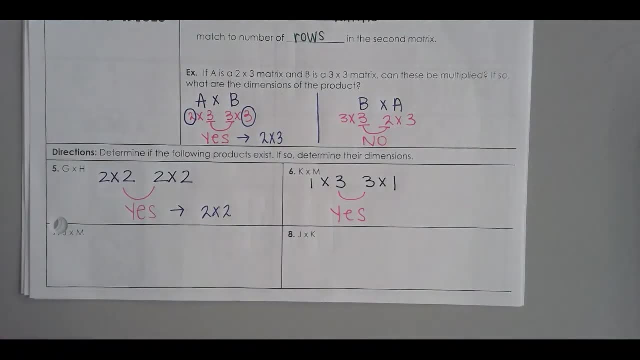 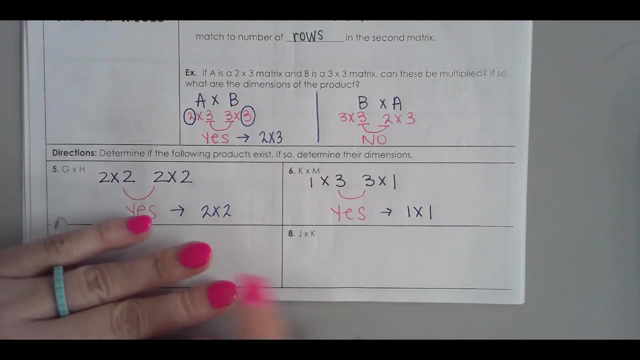 M is a Three by one. Does it work? Yes, it does. What size will my answer be? One by one. Guess what That? if this was the question I gave you, to actually multiply out, it's going to be pretty. 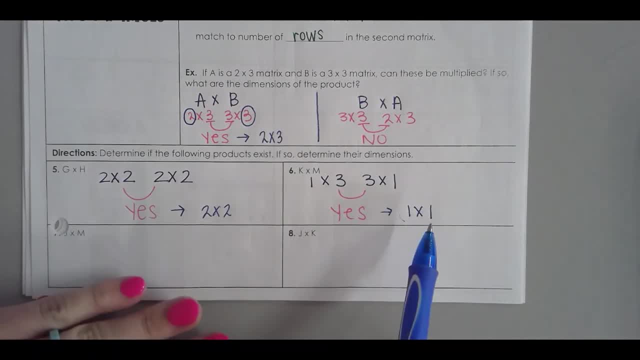 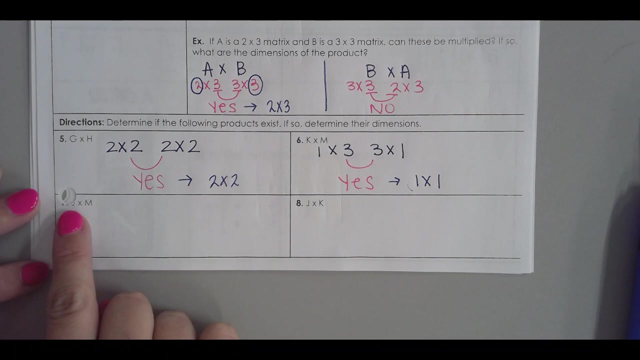 easy, Because your answer only has one element in it: A one by one is one number. Those would be the easiest problems to do. Um, is that J Is somebody else's? Is it J? Sometimes the hole punches aren't on the same spot. 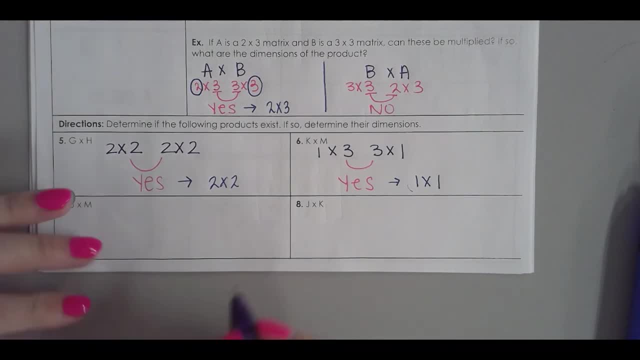 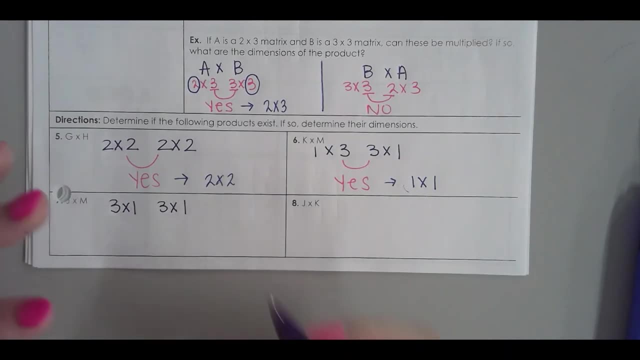 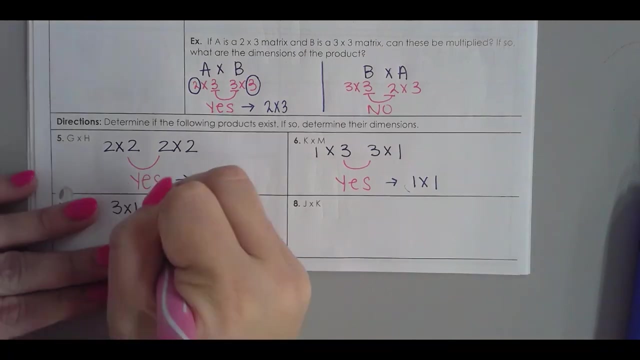 So J is a Three by one, Three by one And M is a. You would think of course I can do negative seven times six, Negative eight times, negative two, But actually it does not work, You can't do it. 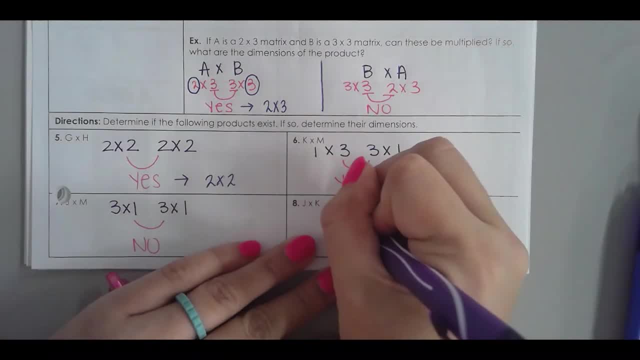 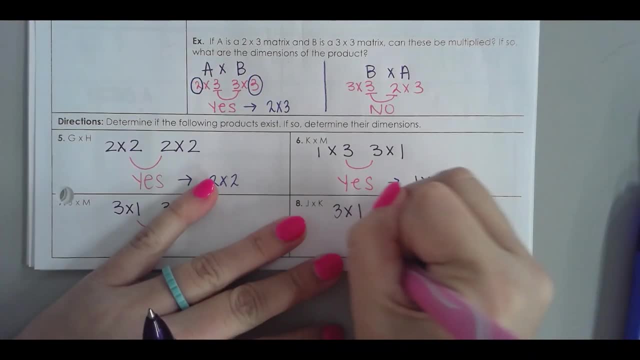 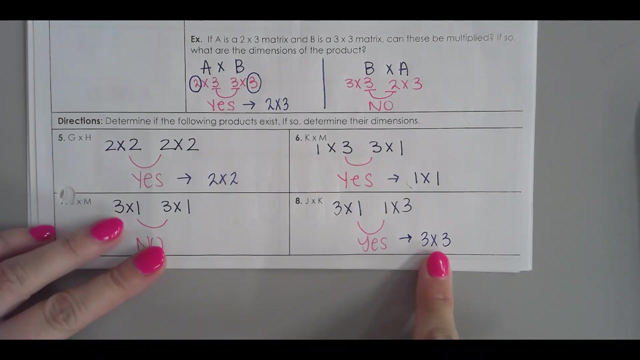 J, we said was a three by one And K is a One by three, It works. My answer is going to be a Three by three, That one. So for a question like this you would have to do: 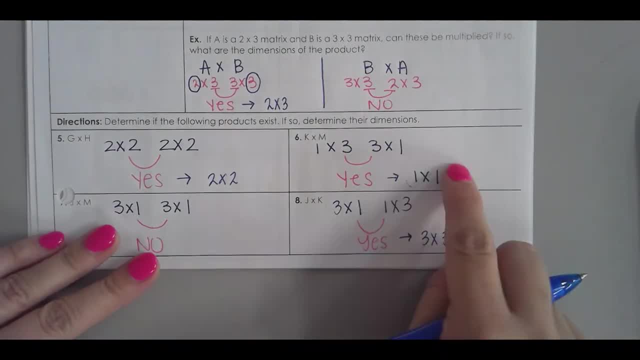 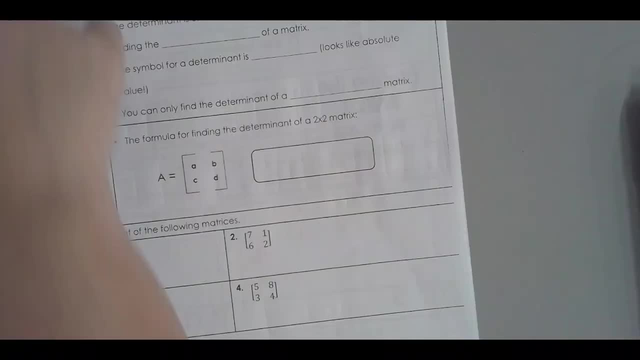 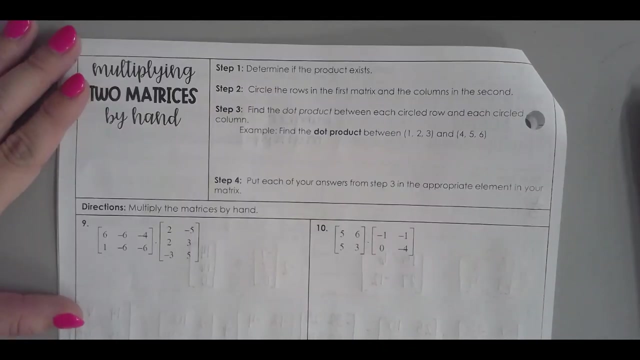 nine calculations because there's nine elements. You would only have to do one calculation because there's only one element. Now we're going to see how to actually do it. If I give you two matrices to multiply, go ahead and see if it's even possible. 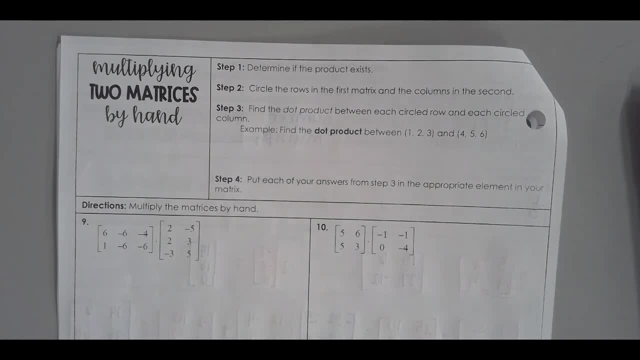 If it's not, you're going to waste some time. You're going to get down to it and start working it out and then realize you can't even do it. Alright, The number, it's just. it has to do with the numbers. 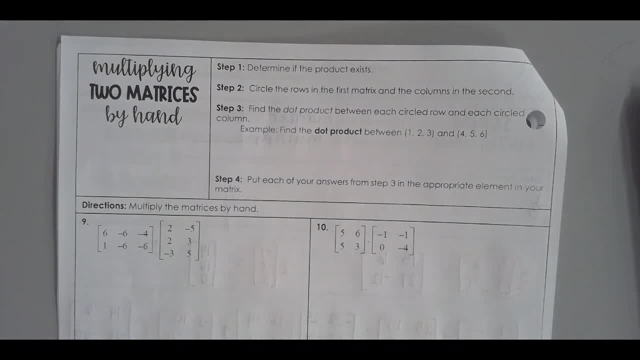 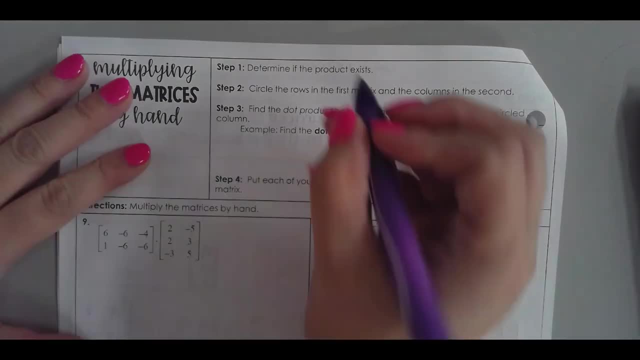 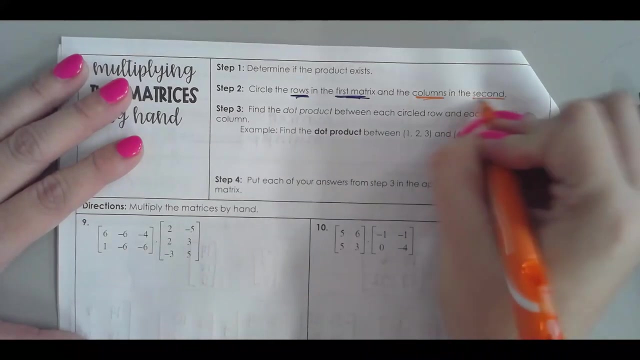 So step two is just a way to kind of keep you organized, help you not make mistakes. Circle the rows in the first matrix and circle the columns in the second, And we will label them row one, row two, column one, column two or however many there are. 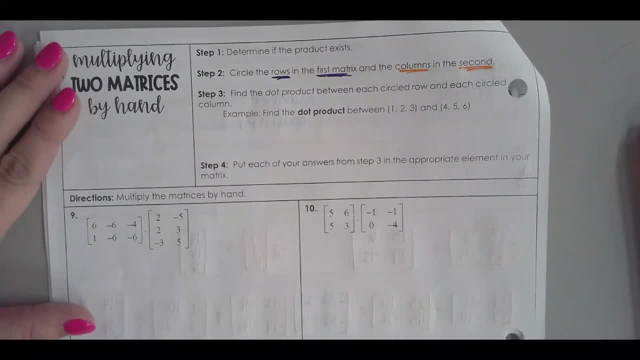 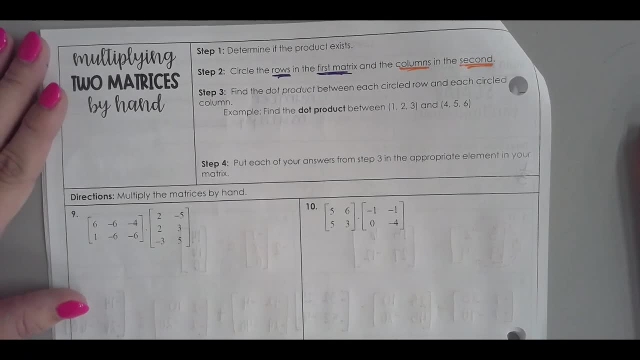 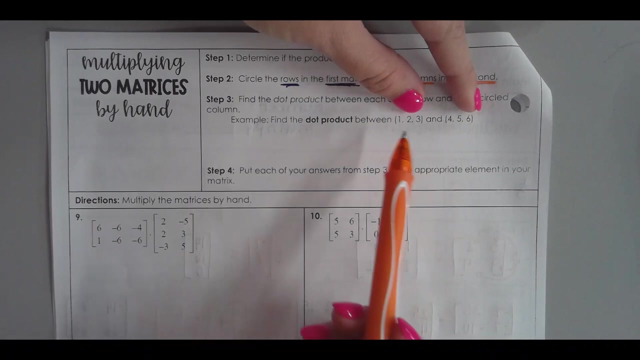 And then the actual calculation comes in. next, You're going to do something called the dot product, And you don't know what that is yet, but it's not hard. So, the dot product: what you do if you have two. 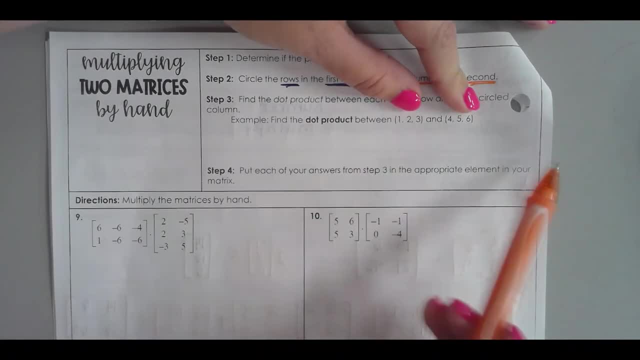 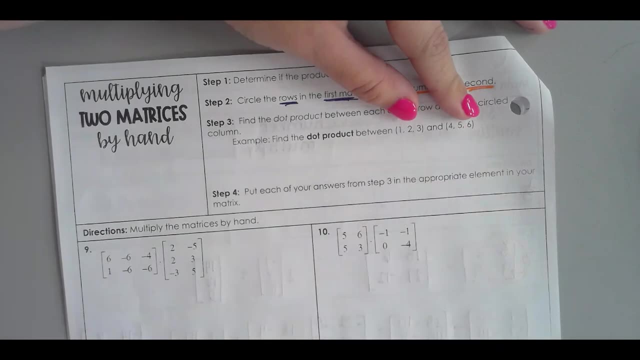 lists of numbers. your lists have to have the same amount of numbers in them, Like this one has three numbers, that one has three numbers- A question where the dimensions don't work out like a. no, you wouldn't have the same amount of numbers in each group. 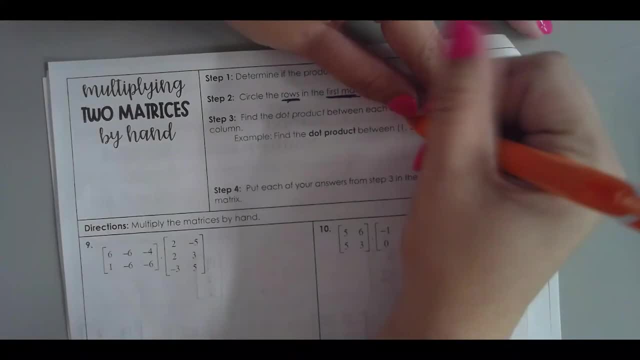 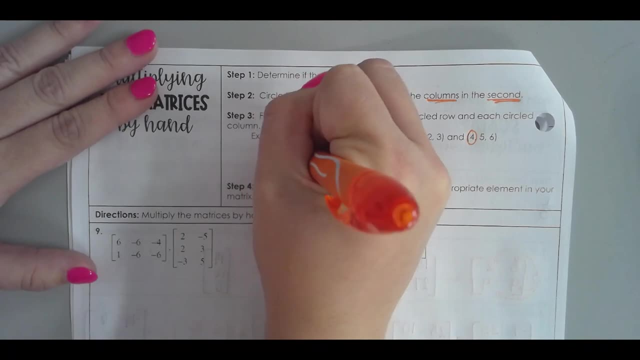 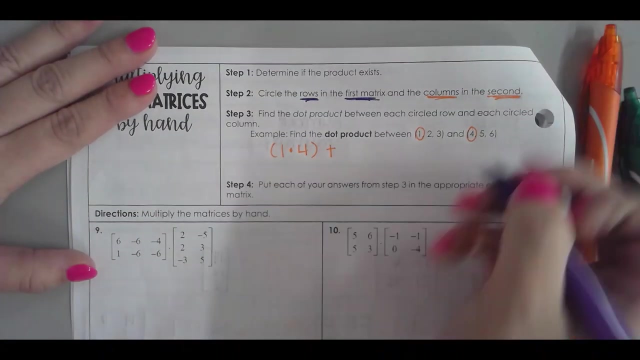 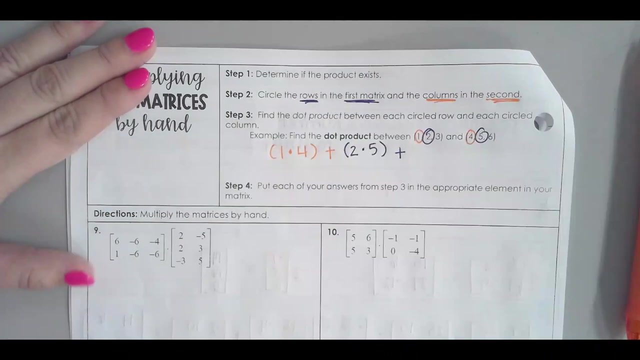 That's why it doesn't work. So the dot product: you take the first two numbers and you multiply them, So one times four plus. and then you take the second two numbers and multiply them Two times five plus the third Three times. 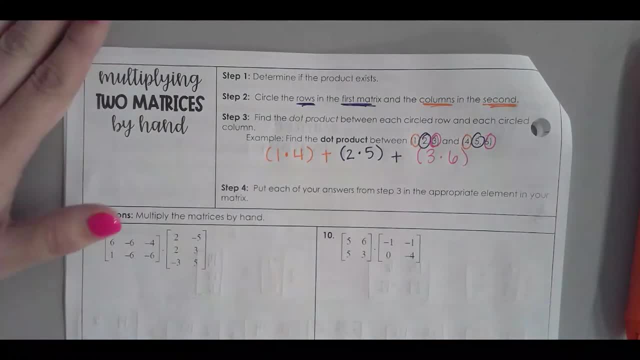 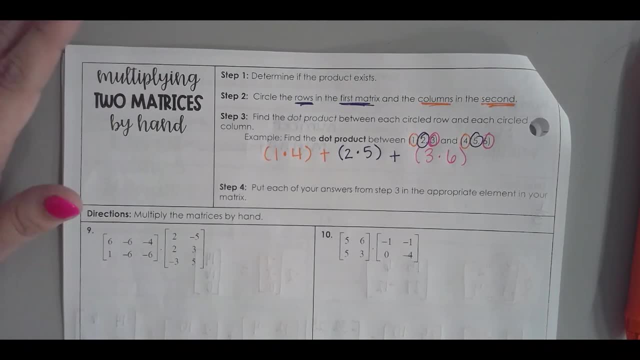 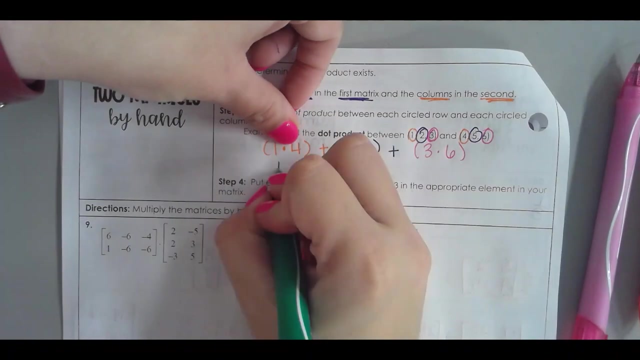 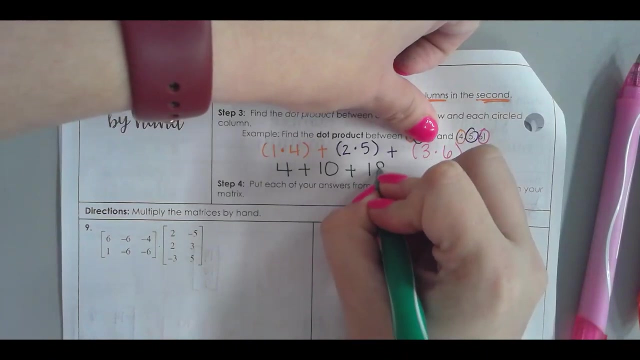 six. So you multiply the first two numbers, multiply the second numbers, multiply the third numbers and then add all that together. So what is one times four Plus two times five Plus three times six is eighteen, And that gives you what. 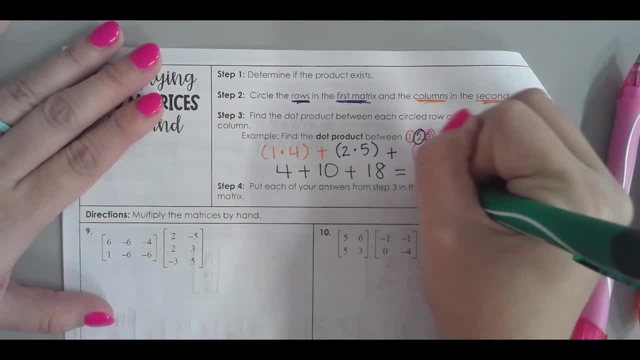 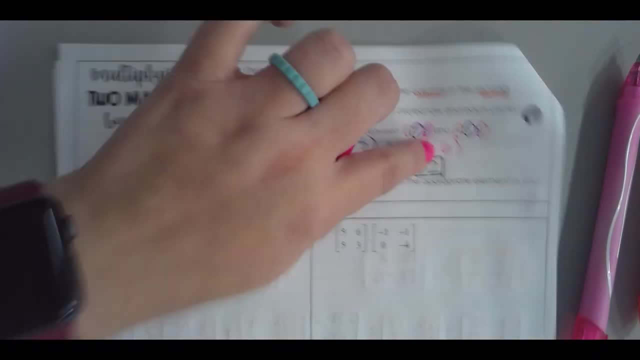 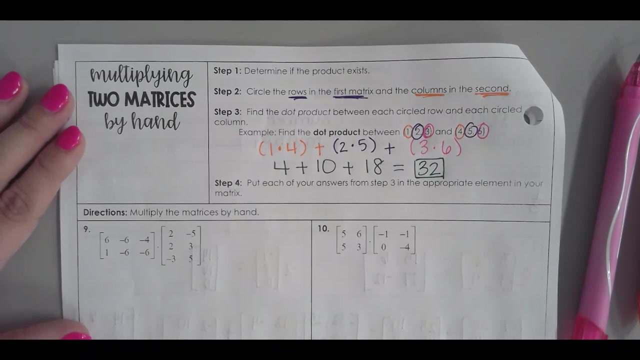 Thirty-two, And you have to do that For every element. that's in your answer. that's how many times you have to do this. So let's get into a real example. So number nine: First off, let's just go ahead and check to. 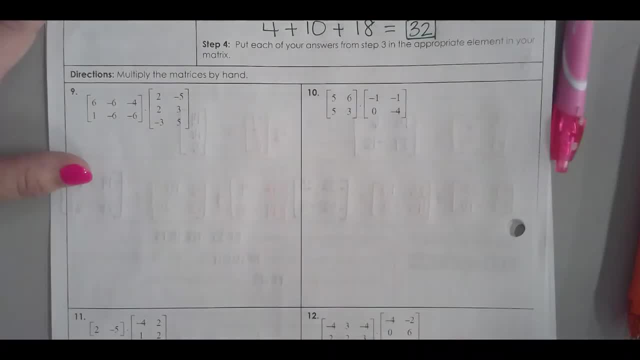 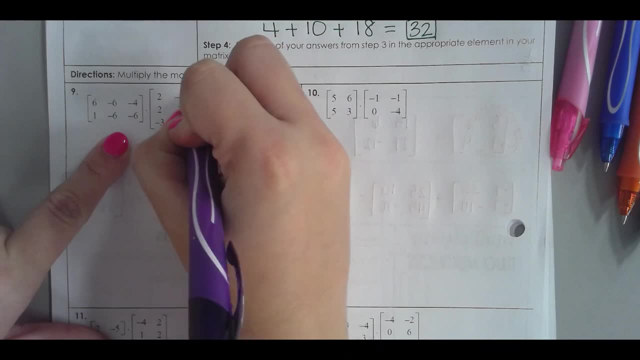 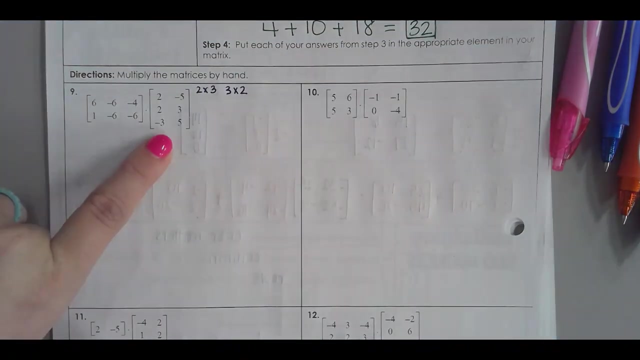 see if it works. So the first matrix is a what Two by three, And the second one is a three by two. Does it work? Yes, it works, And my answer is going to be a what Two by two, Those outside numbers. 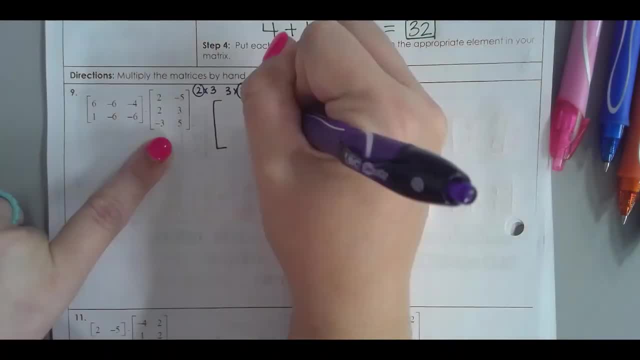 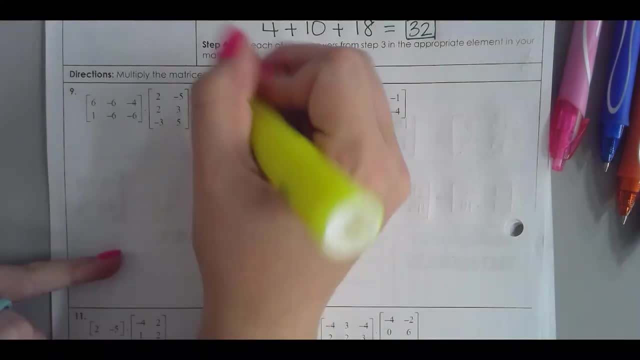 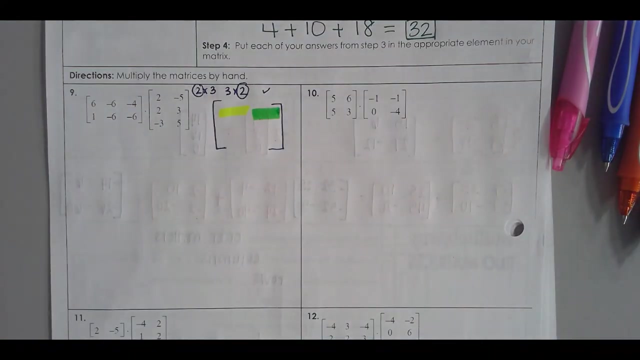 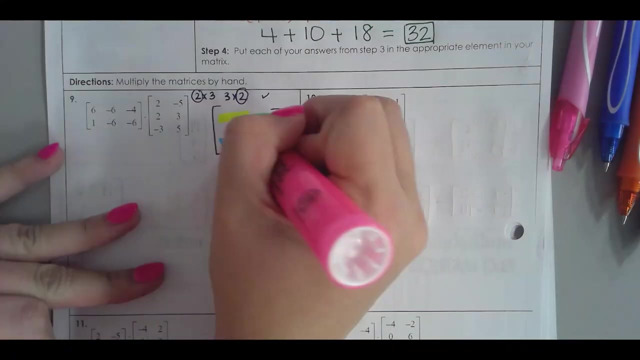 tell us. So I'm going to go ahead and make a matrix that's going to fit my answer And you don't have to do all this highlighting and stuff That just helps visual people. So my answer is going to be a. 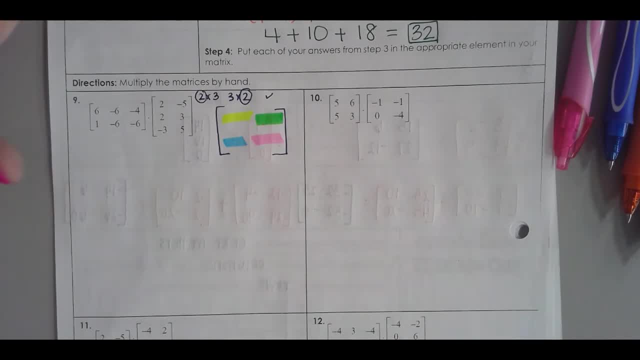 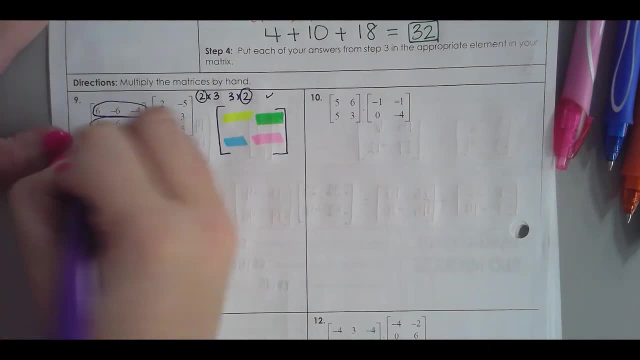 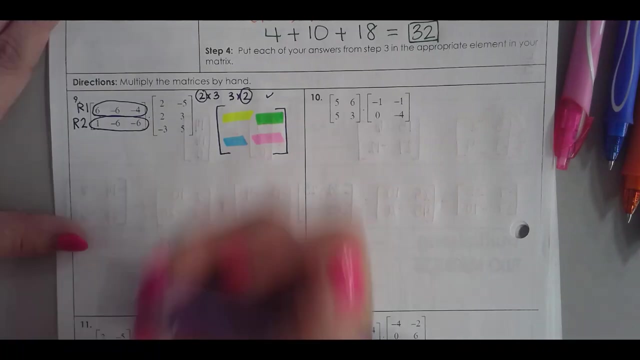 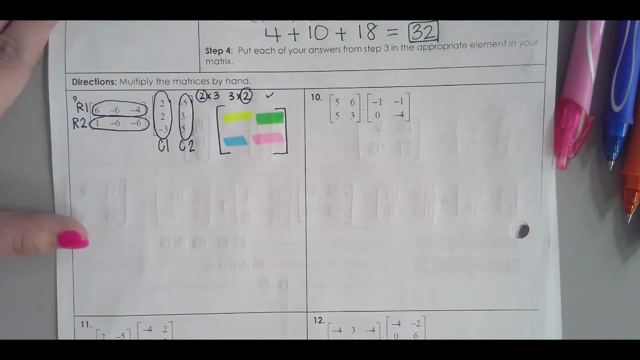 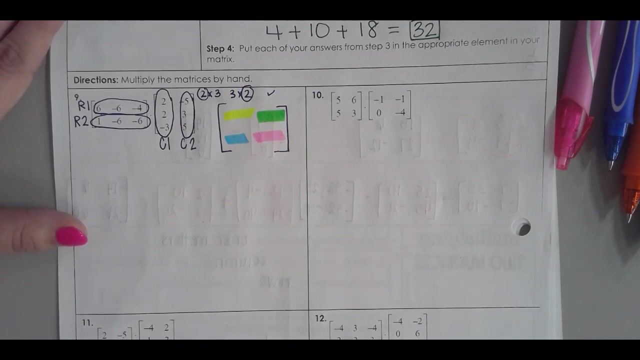 two by two. Let's circle the rows in the first matrix- Row one, row two- And circle the columns in the second Column one, column two. In my answer, this blank that I've highlighted in yellow, what row is that in? 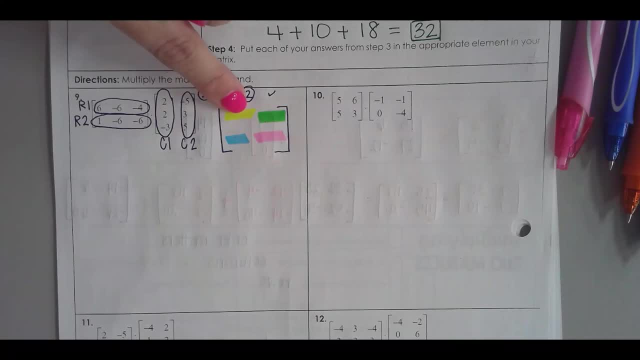 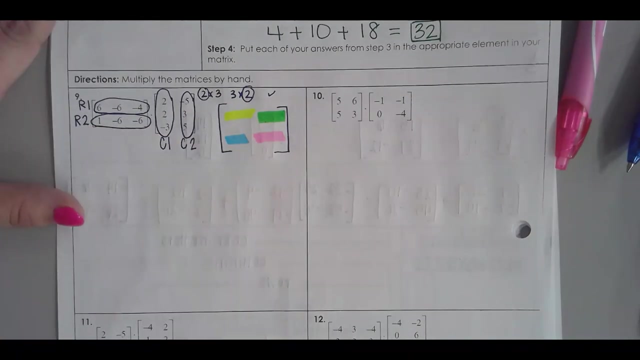 Row one. What column Column one? So you're going to do the dot product between our row one and column one And that answer goes in that blank. So row one, the one that I have circled and labeled row one. 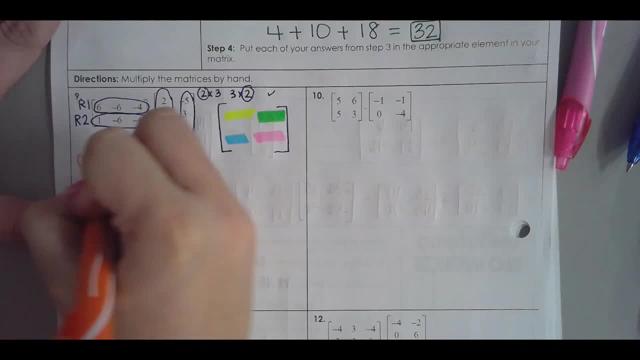 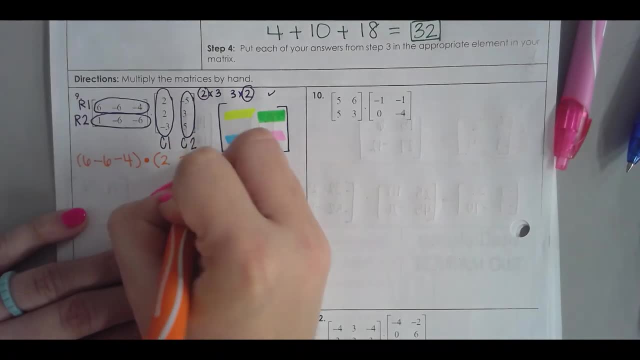 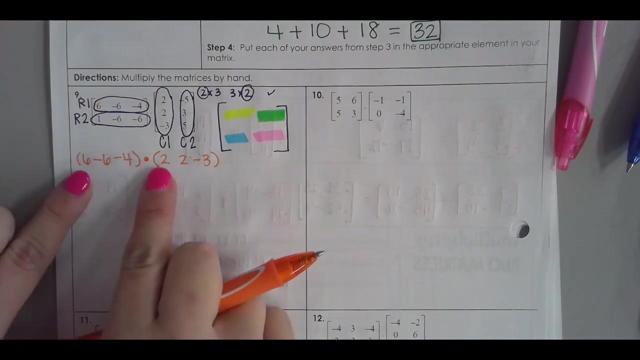 six negative, six negative four. I'm going to do the dot product with column one, Two, two negative three And you don't have to show the six times two. You don't really have a lot of room to do that. 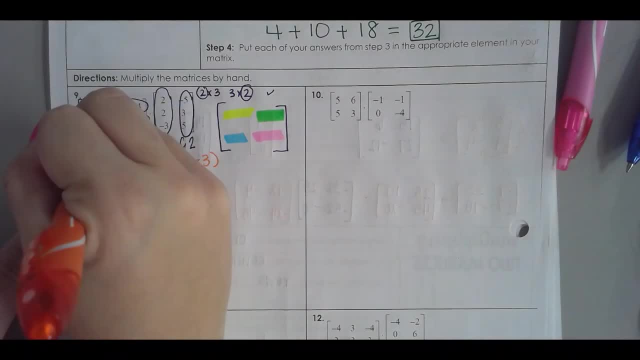 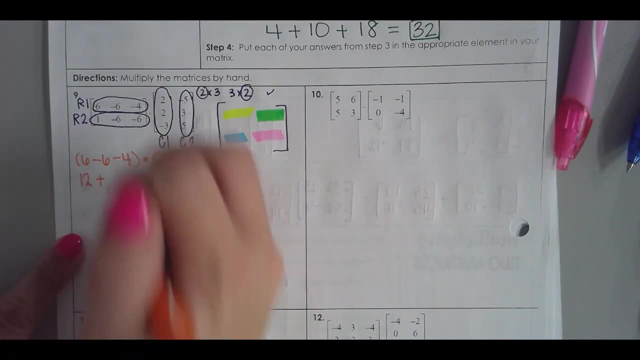 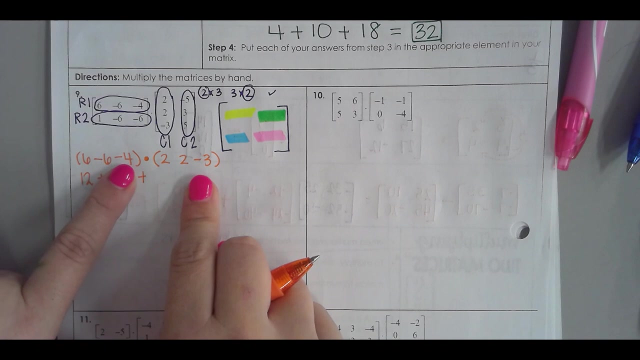 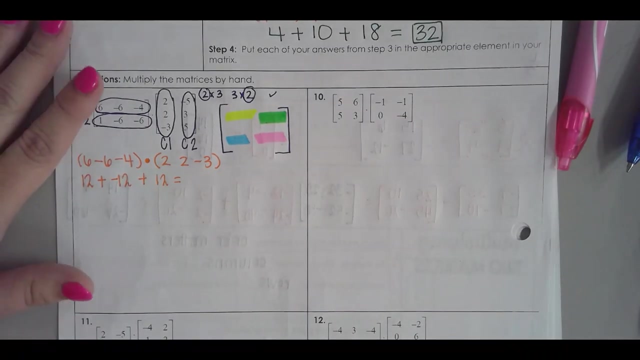 So what is six times two, Twelve Plus what's negative six times two? Yeah, negative twelve Plus negative four times negative, three Positive twelve, And what do you get when you add all three of those numbers together, Twelve. 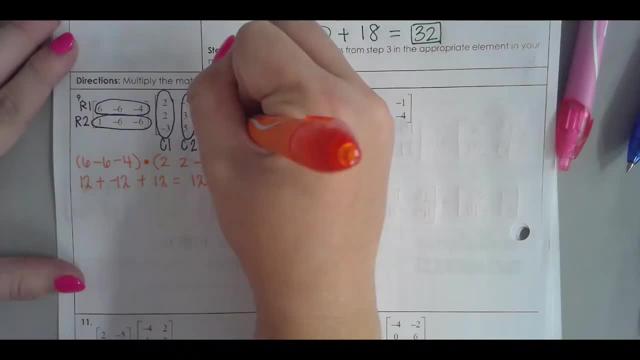 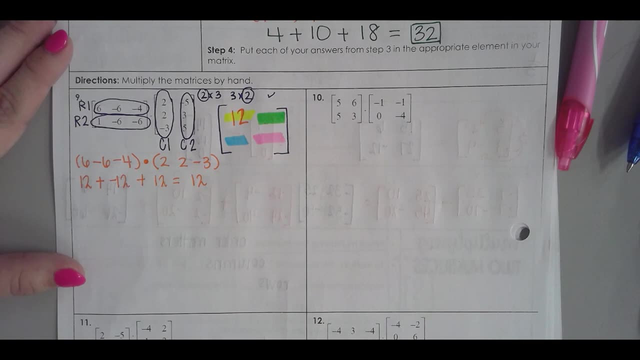 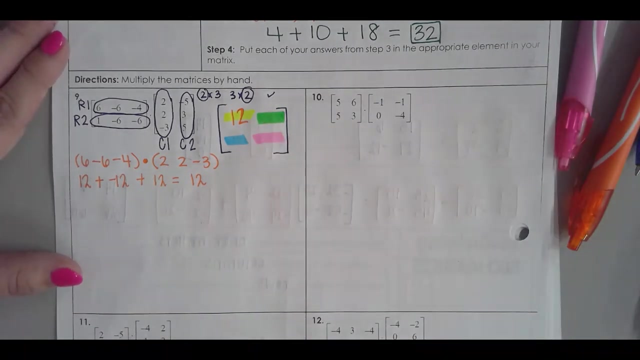 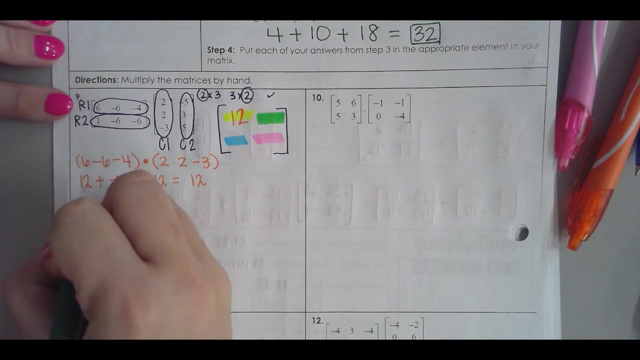 It is twelve. That's funny And that answer goes right there. Now this next element is in row row one, column two. So I'm going to do the dot product between row one and column two. So my row one, six. 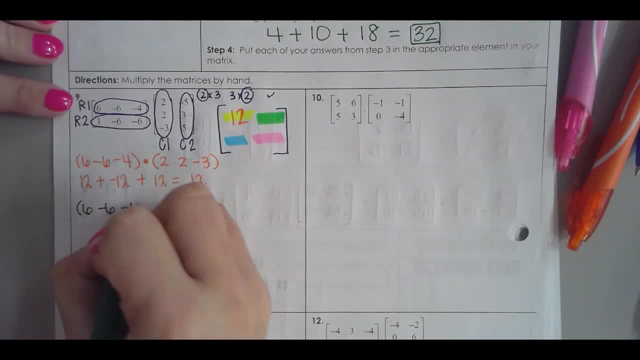 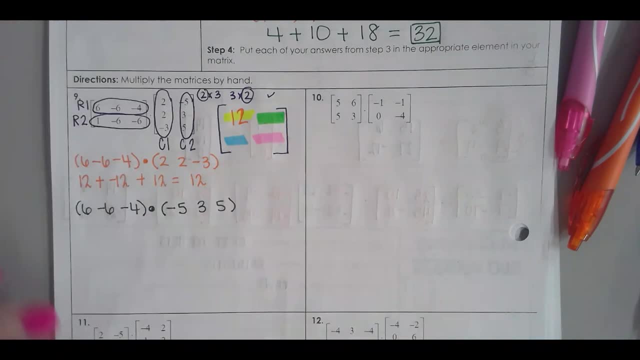 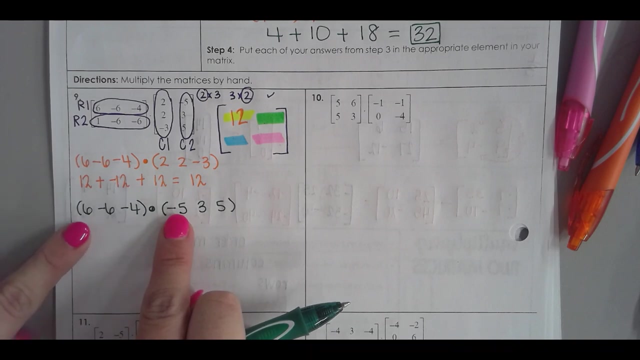 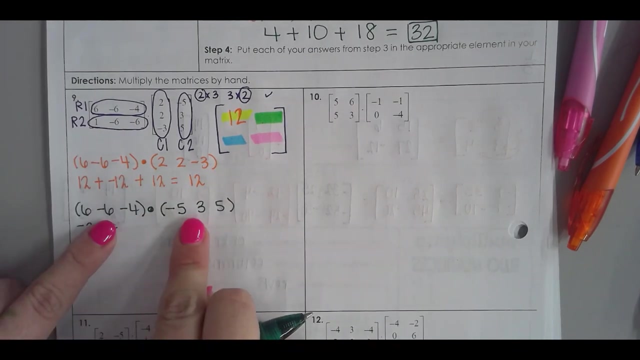 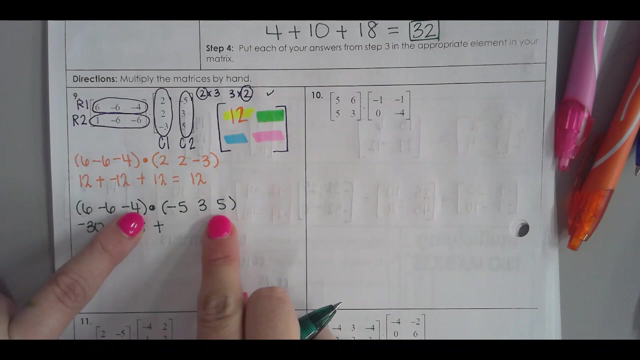 negative six negative four. Column: two: negative five: three, five, Six times negative five is negative. thirty Plus negative six times three: Negative eighteen. Negative eighteen Plus negative four times five: Negative twenty. And this gives you: 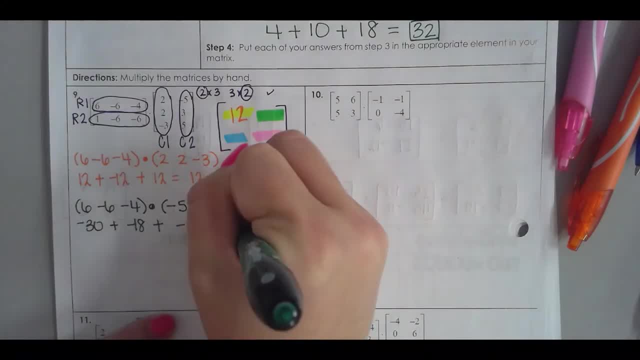 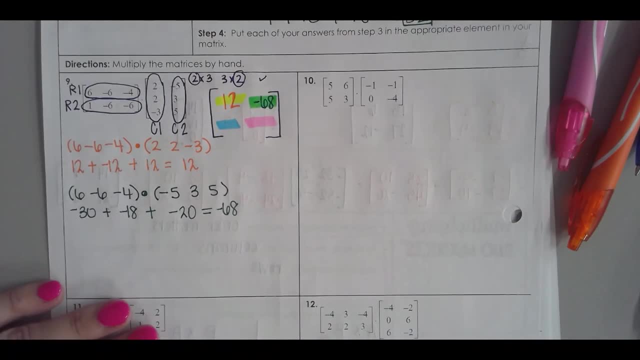 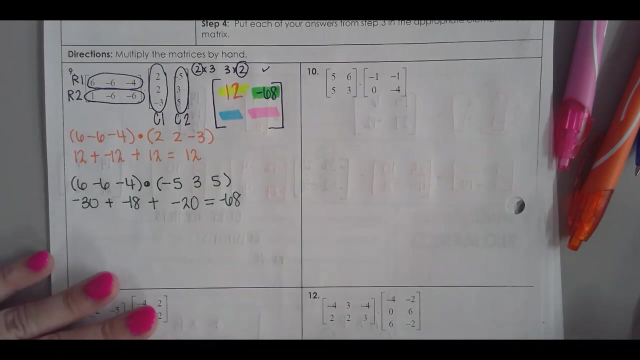 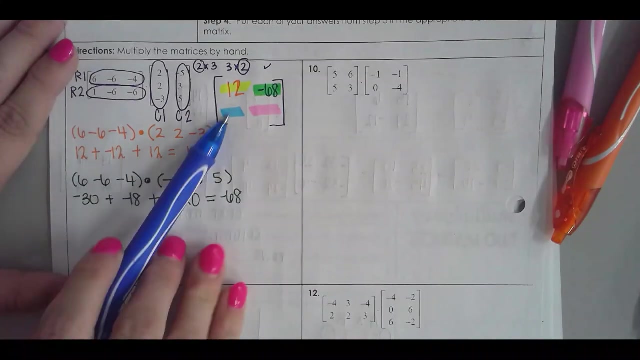 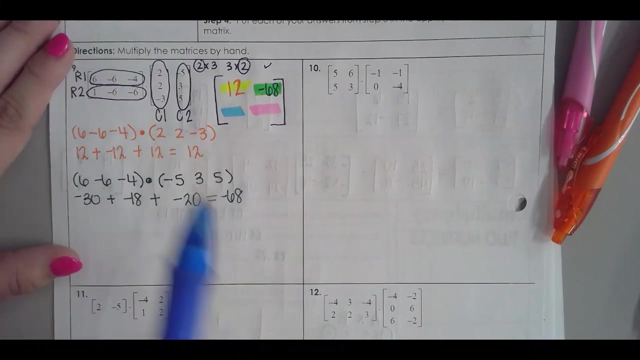 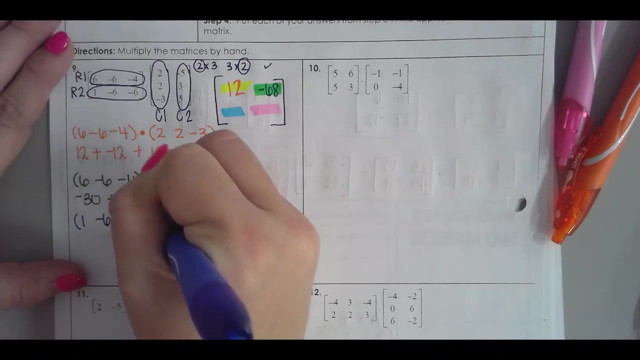 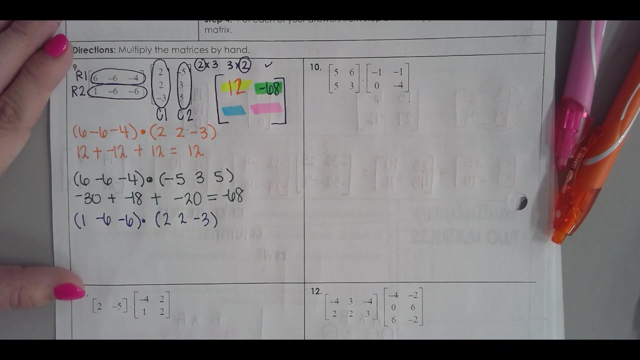 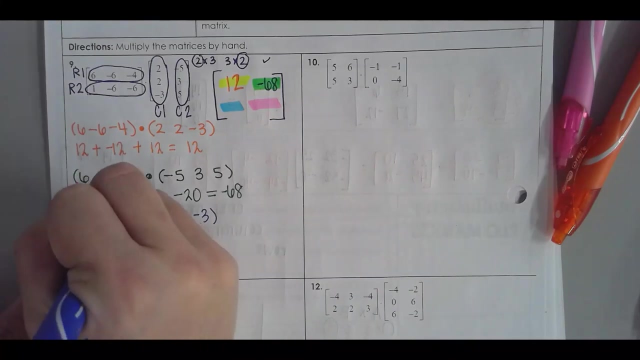 negative sixty-eight. Okay, Now my next one, the one I have in blue. That one is row two, column one. So row two dotted with column one, One times two is Two Plus negative six times two. 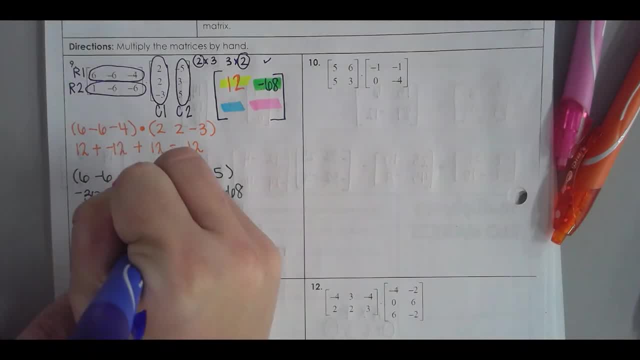 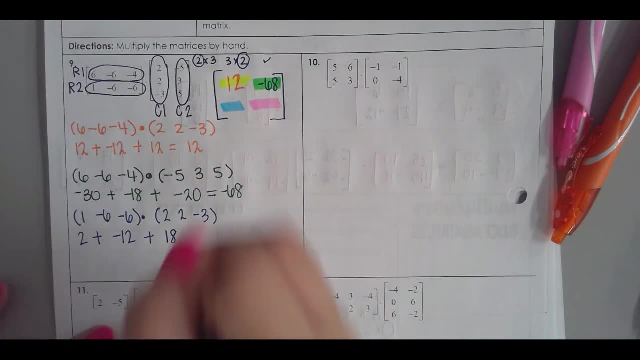 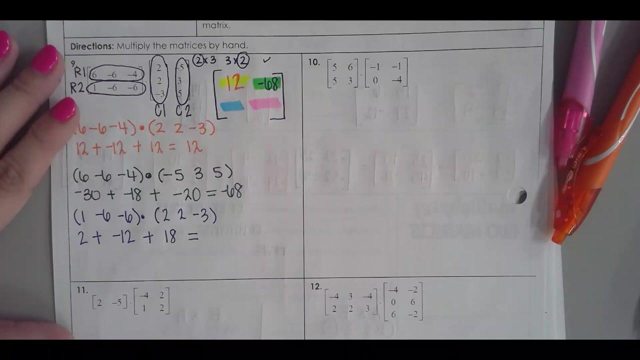 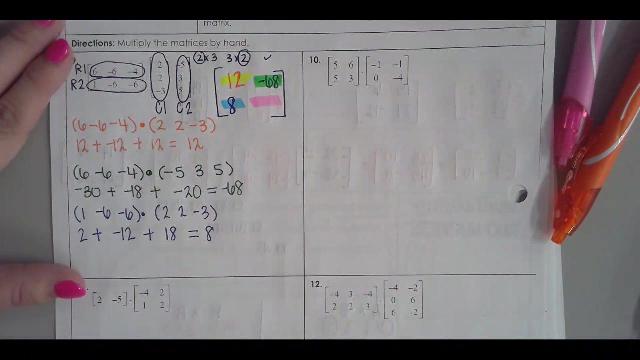 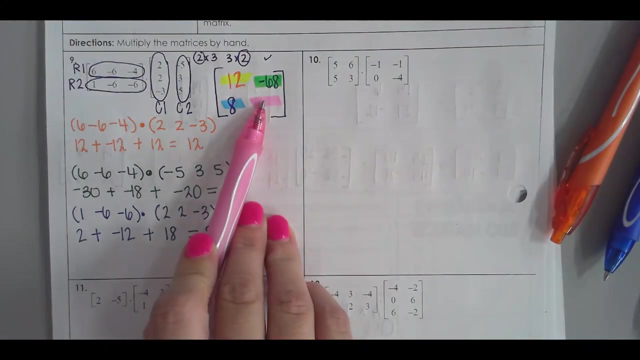 Negative twelve Plus negative six times negative three, Positive eighteen, And when you add those together you get eight. The last one is in row, column two, So one negative six, negative six dotted with negative five, three. 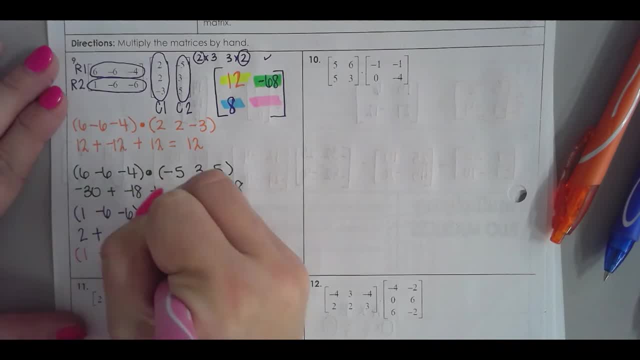 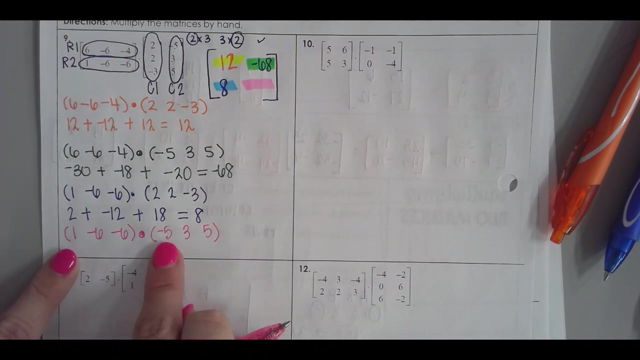 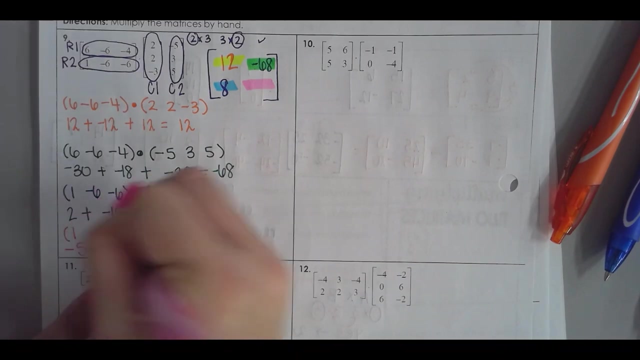 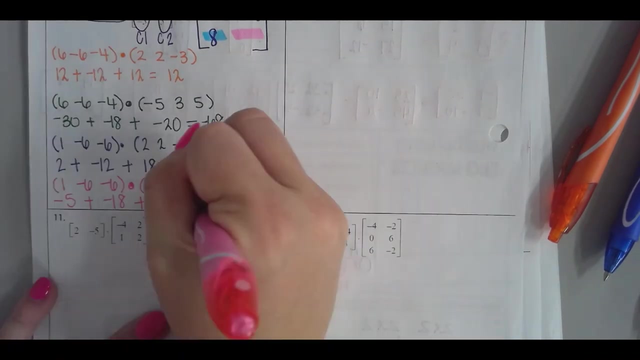 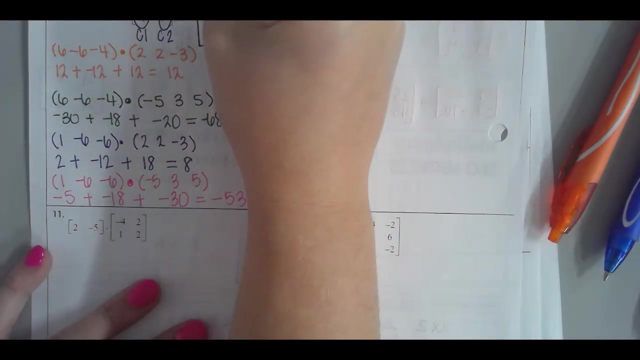 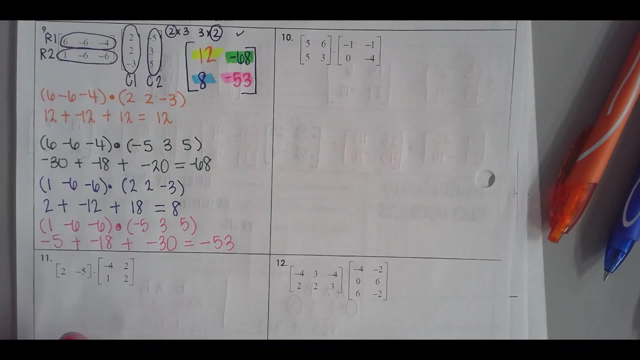 negative, four negative five, three negative, four negative five, One times negative, five is Negative, five Plus negative six times three Plus negative, six times five. Negative, thirty, Negative: fifty-three. First didn't fit you. What does that mean? 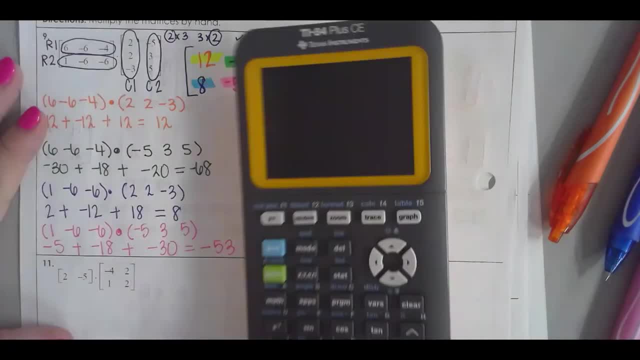 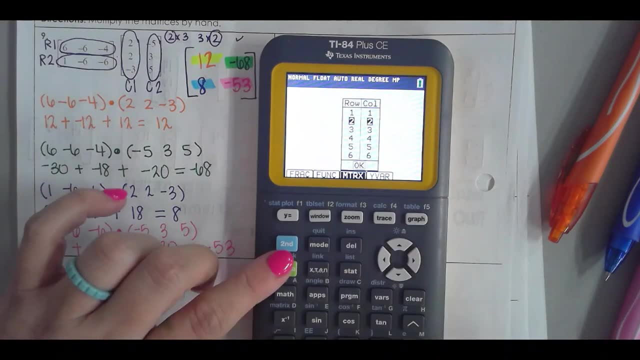 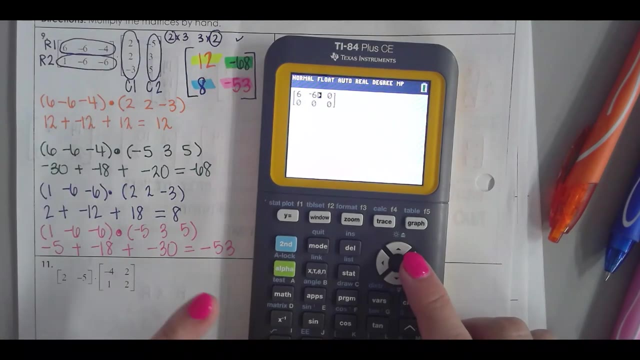 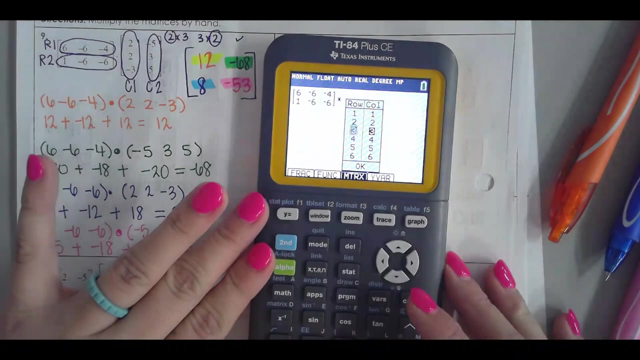 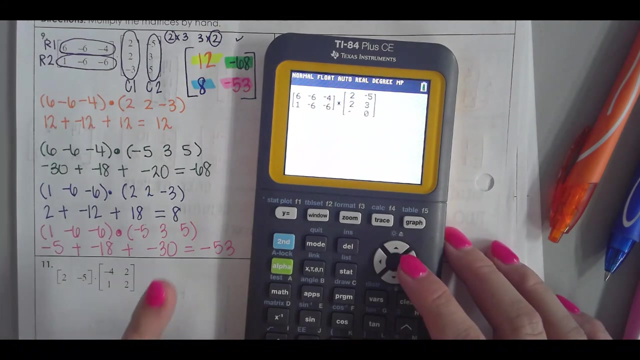 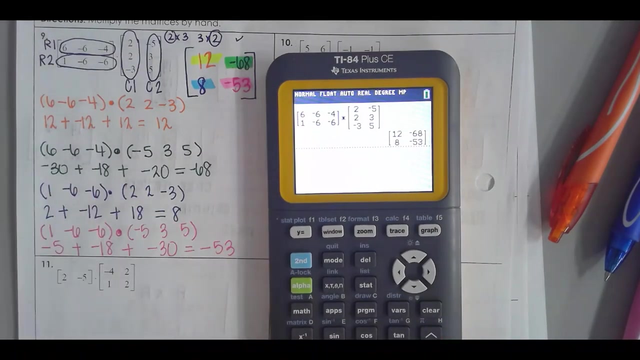 Look at the ochemist online And then you can check your answer On the test. I will expect that you do some of these by hand. Well, 12,. negative 68,, 8, and negative 53.. If one of my four numbers was off, it would be really easy for me to go back and look at the exact space where I messed up and check. just that work. 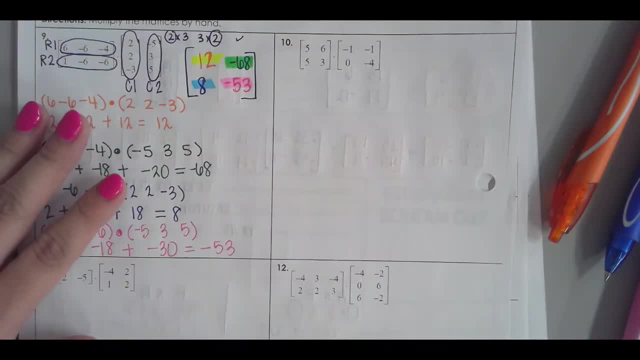 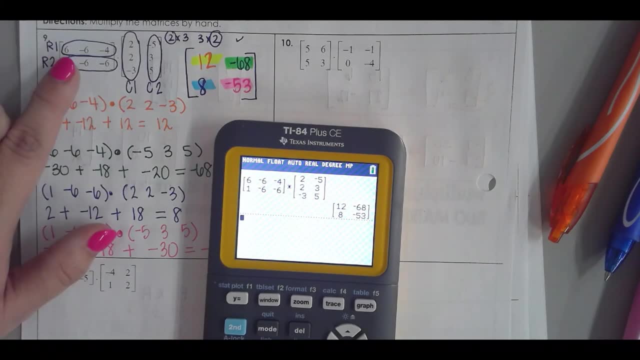 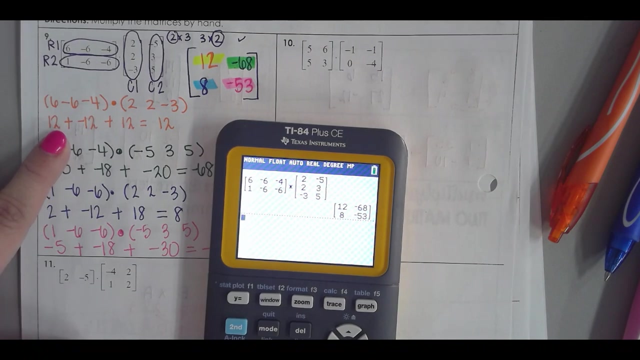 So if I wanted to say, like, which numbers to multiply- I'm just trying to make a note of myself because I forget which numbers, the corresponding numbers, and then add together all the products. Yeah, yeah, I don't know that there's a true word for it. 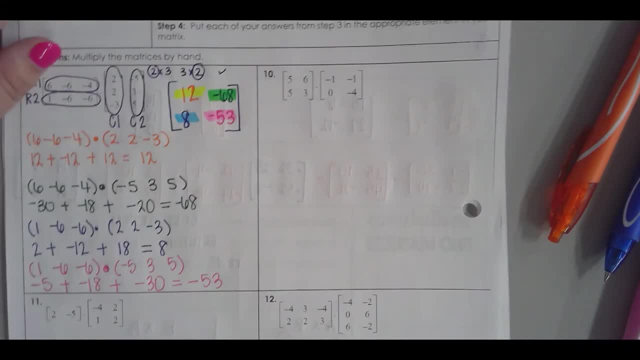 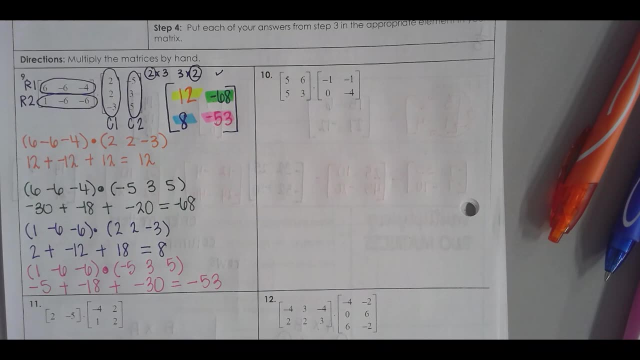 I guess you could say the corresponding elements, maybe All right, number 10.. We have a 2 by 2 and a 2 by 2.. Yes, you can multiply those. What's your answer going to be 2 by 2.. 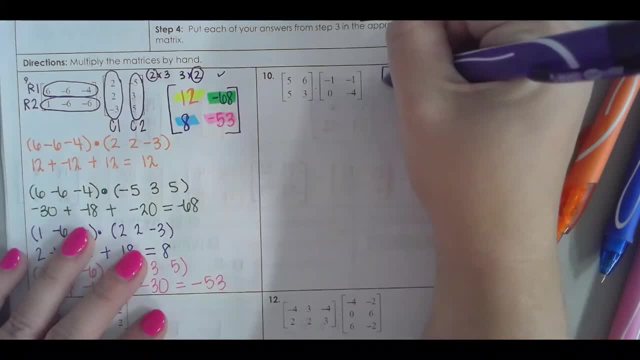 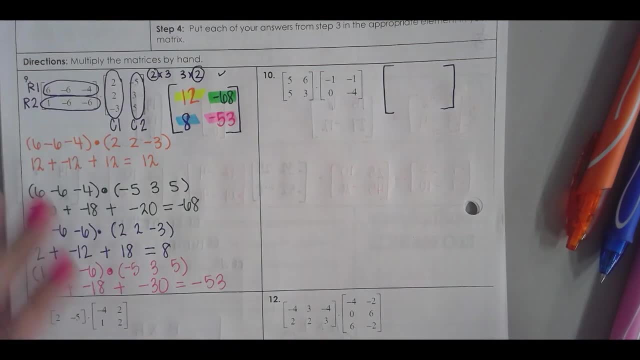 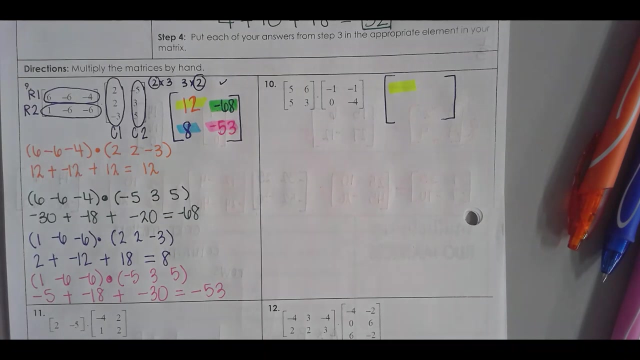 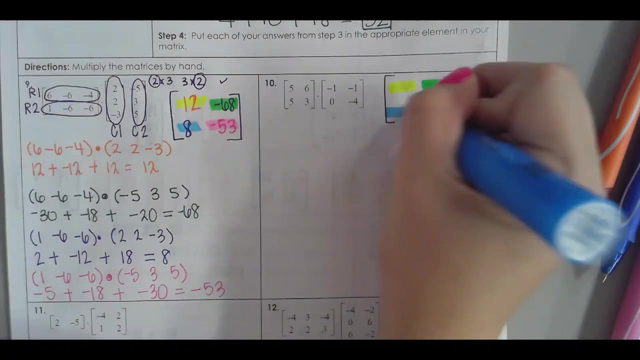 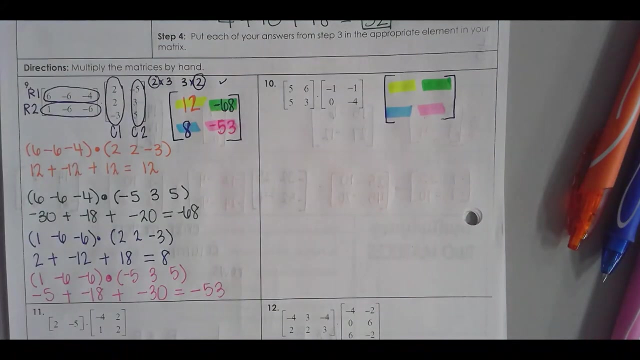 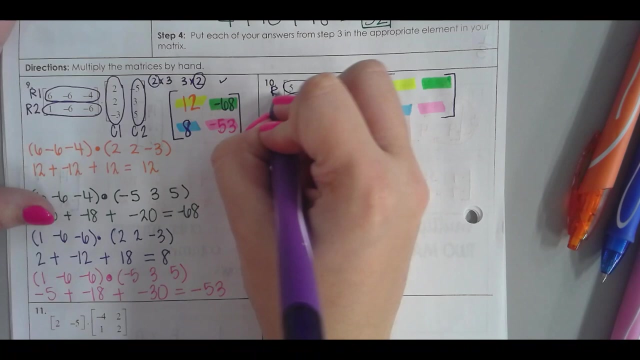 This one will be slightly less work because each dot product we only have, like, two numbers to do. All right, So if we circle the rows and label them, row 1,, row 2, and the columns column 1,, column 2.. 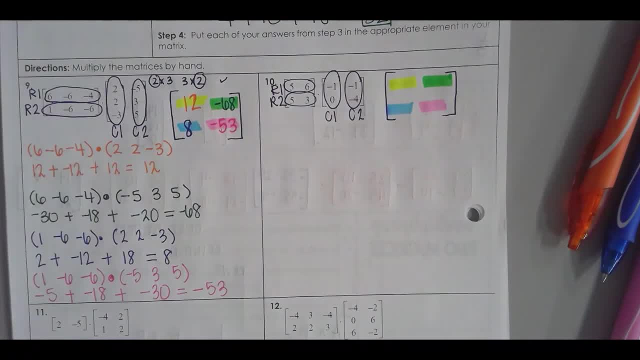 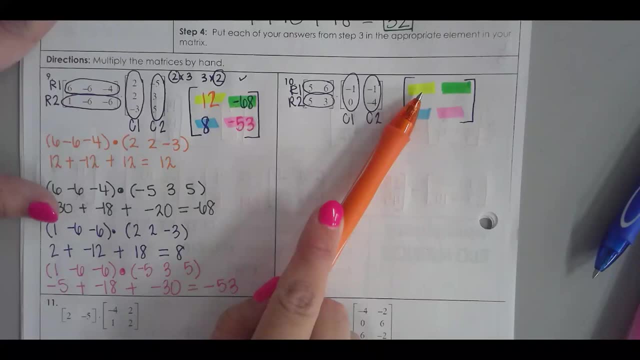 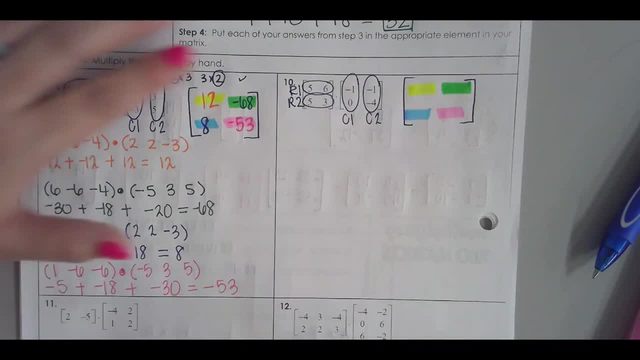 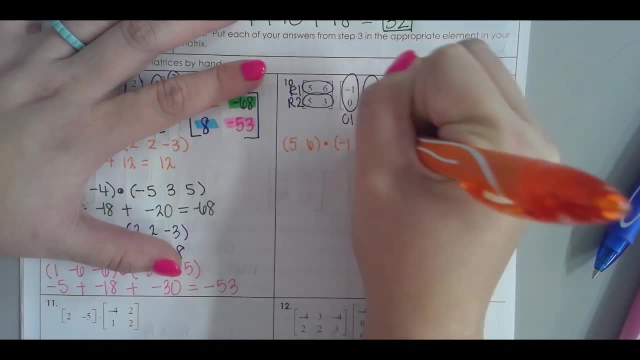 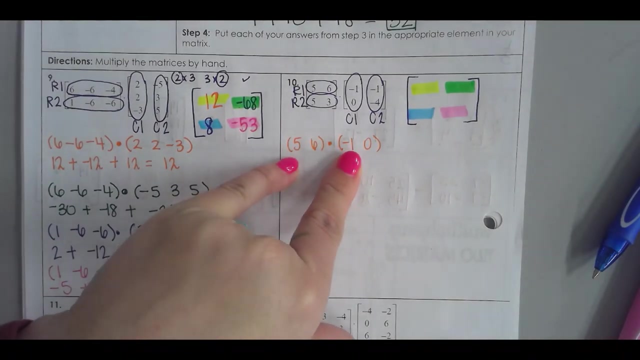 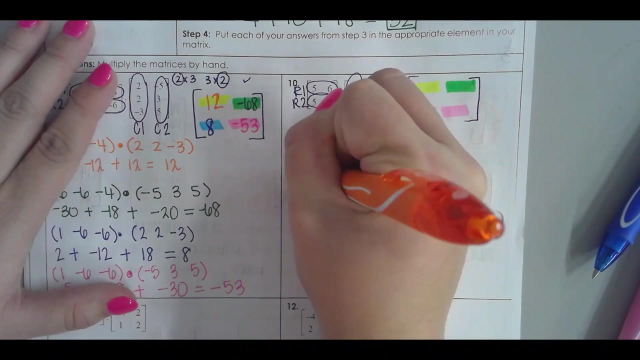 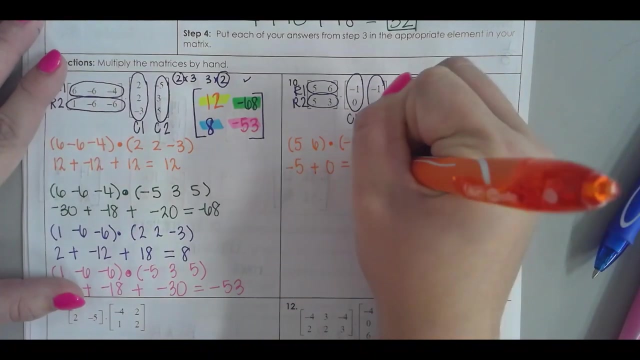 Which column 1.. Yep, row 1 and column 1. We have 5 and negative 1.. 5 times negative 1 is negative 5. Plus 6 times 0, 0,, which gives me negative 5.. 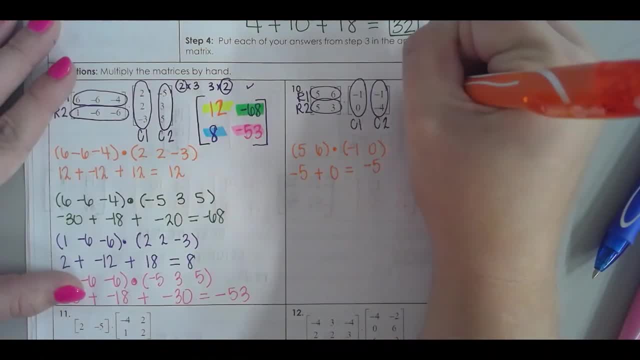 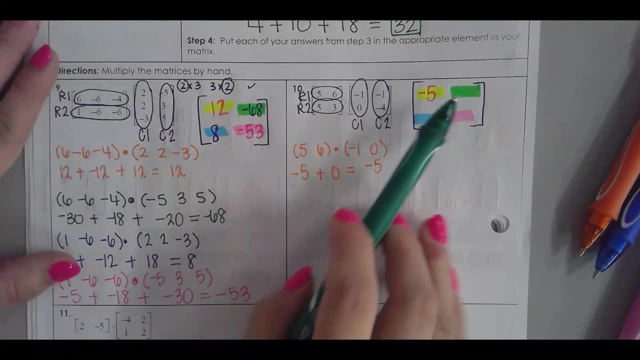 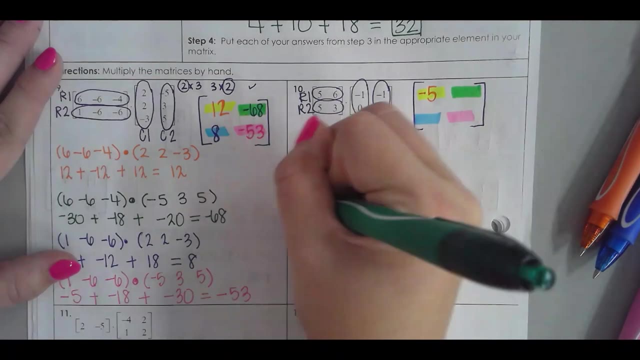 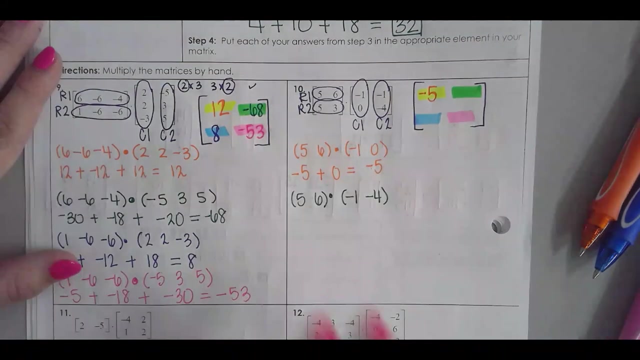 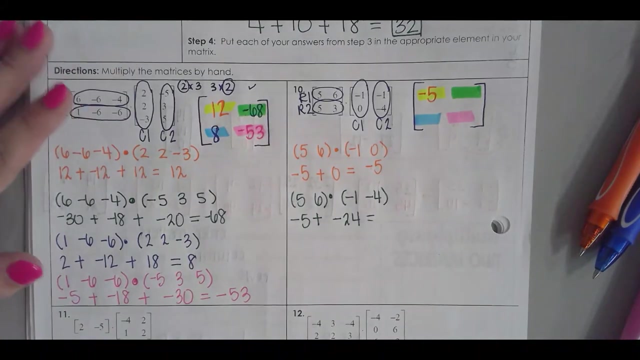 Then we have row number 1 with column number 2. So row 1. And column 2. 5 times negative, 1 is negative 5.. 6 times negative, 4? Negative 24.. Add them together, you get negative 29.. 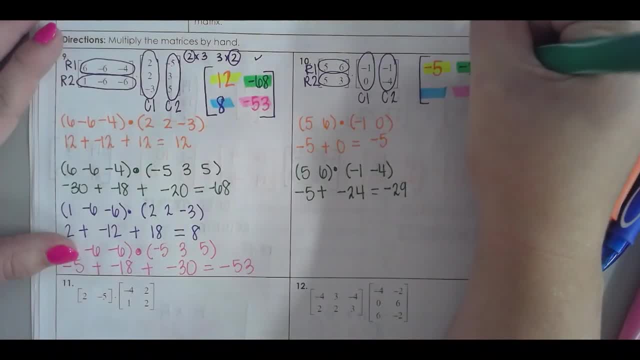 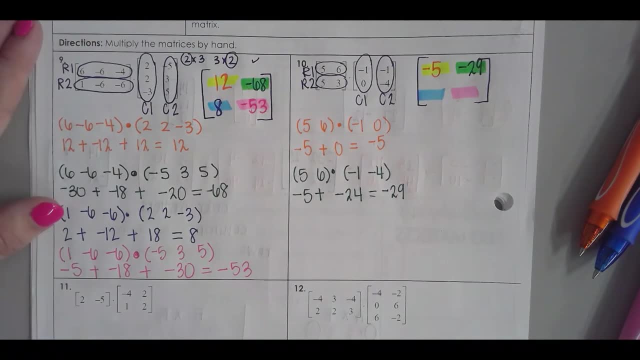 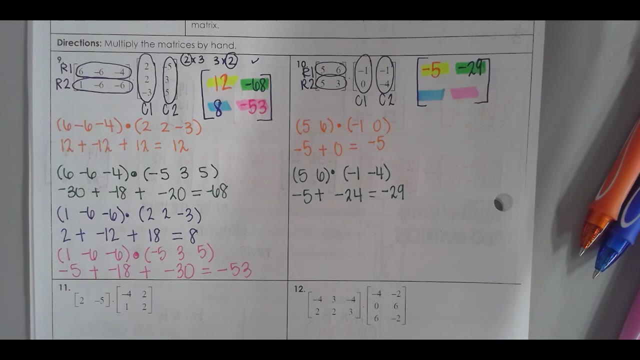 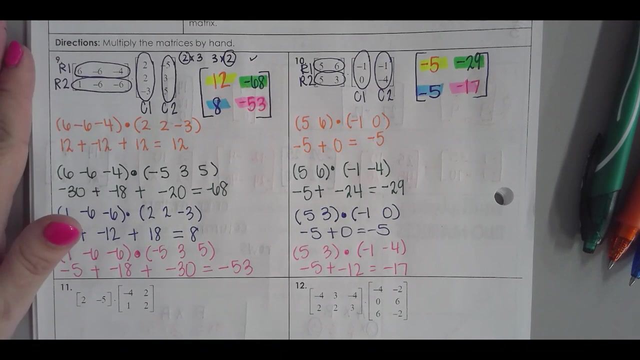 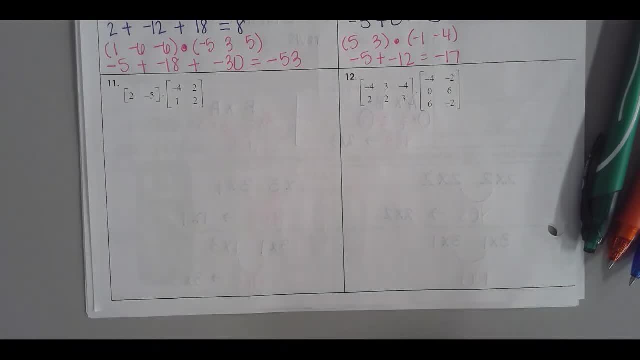 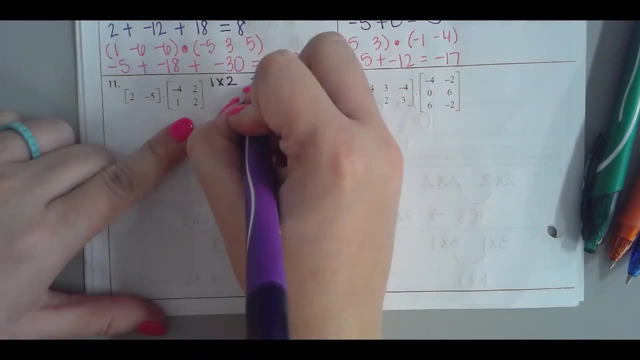 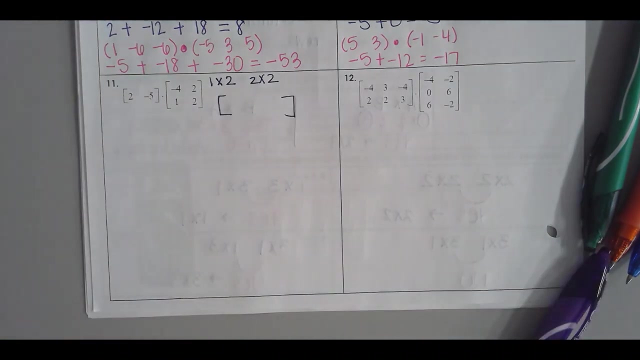 We won't do number 12.. So number 11.. The first matrix is a 11. 1 by 2.. The second one is a 1 by 2.. Circle the rows: There's only one, And then the columns.